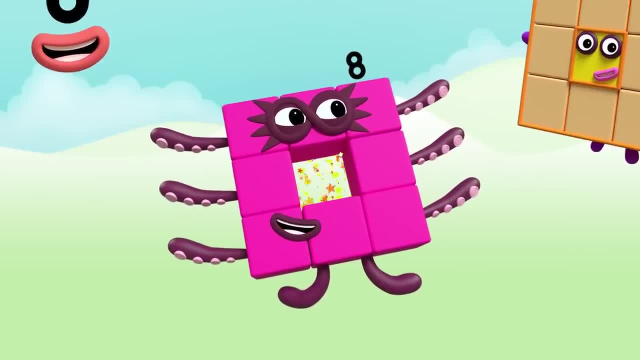 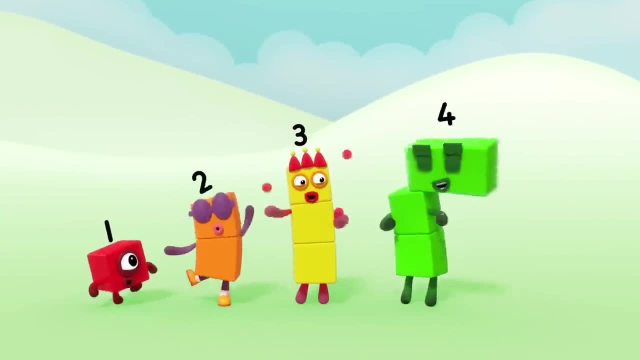 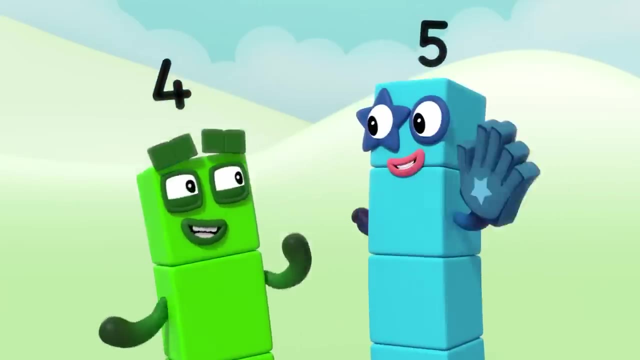 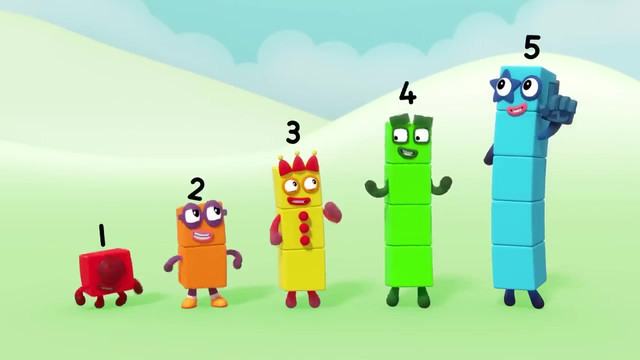 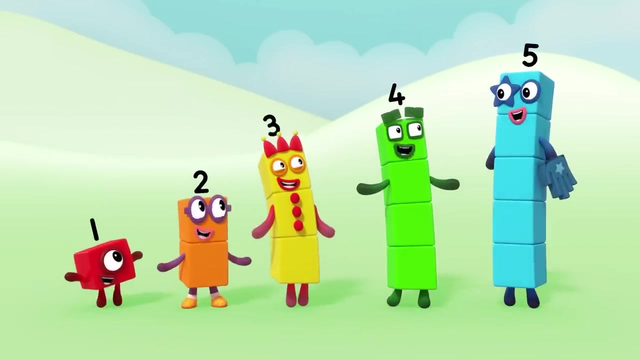 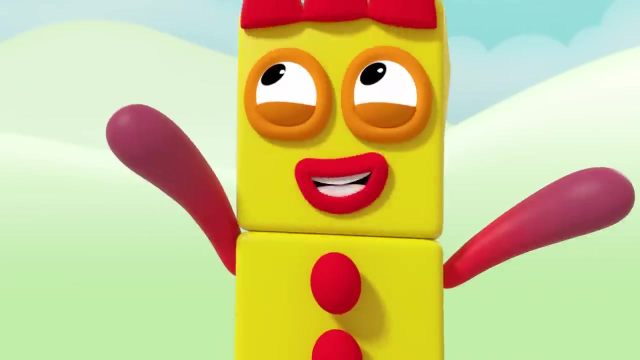 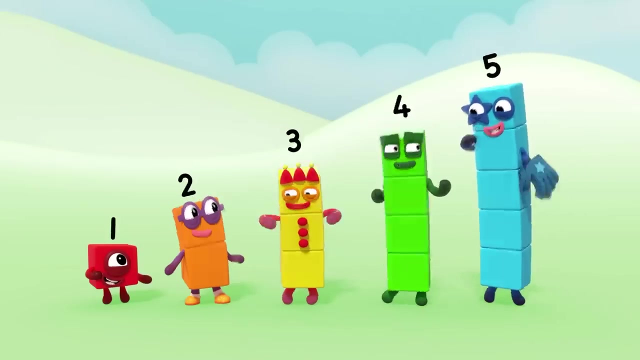 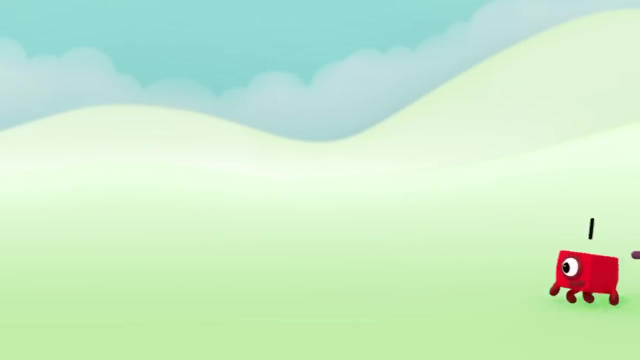 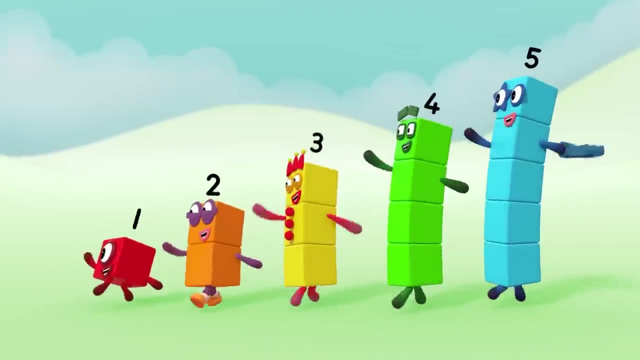 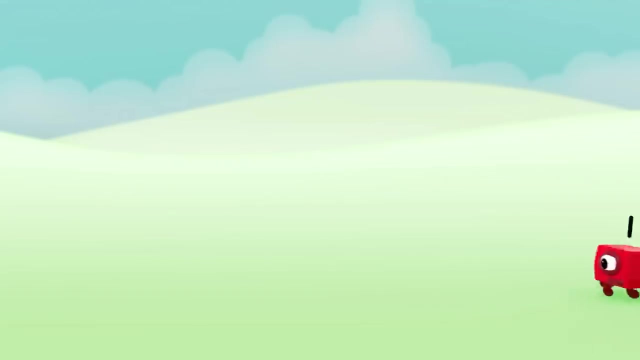 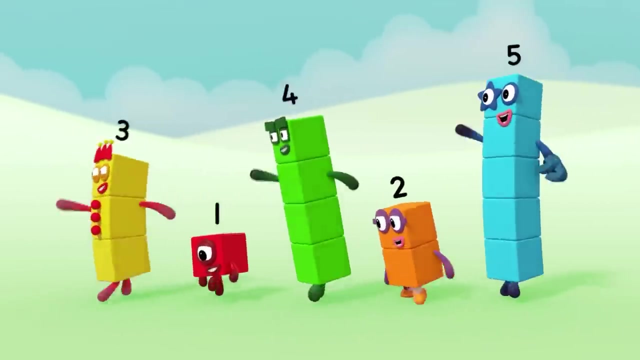 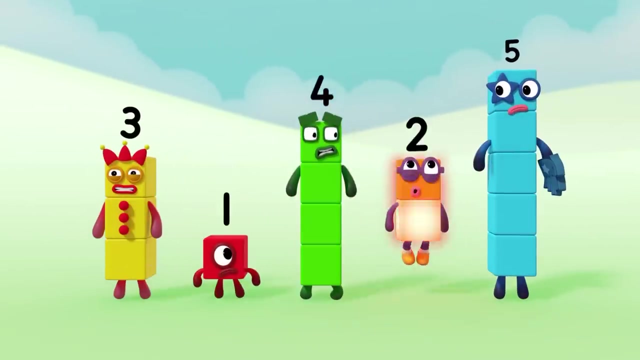 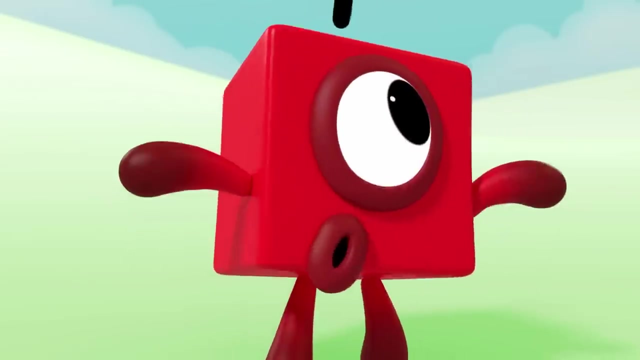 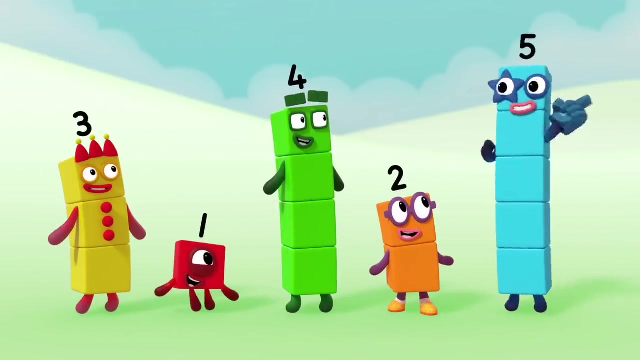 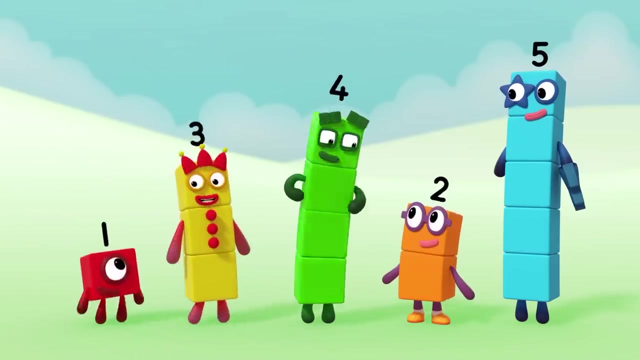 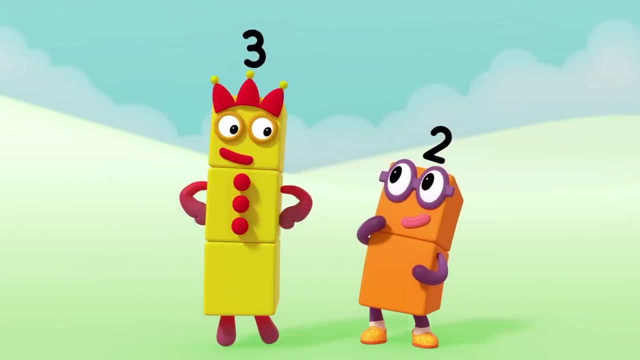 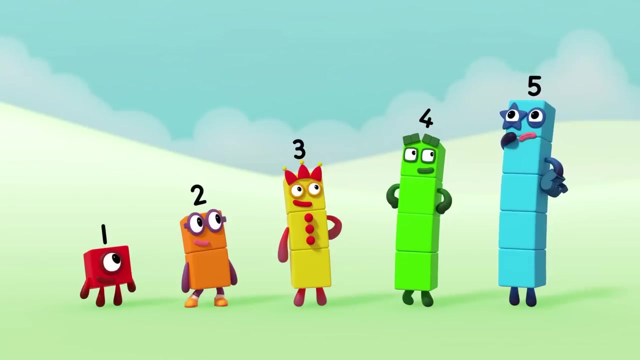 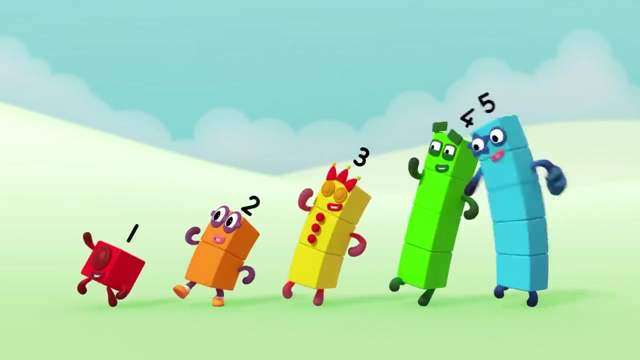 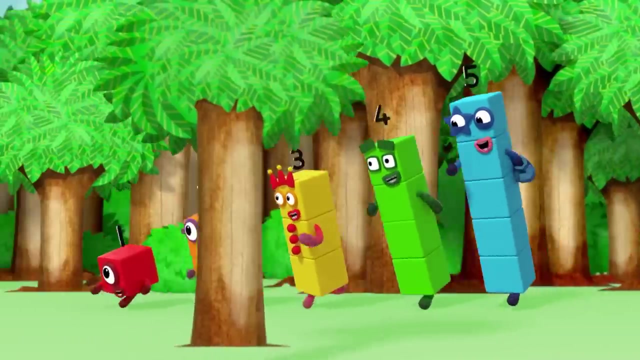 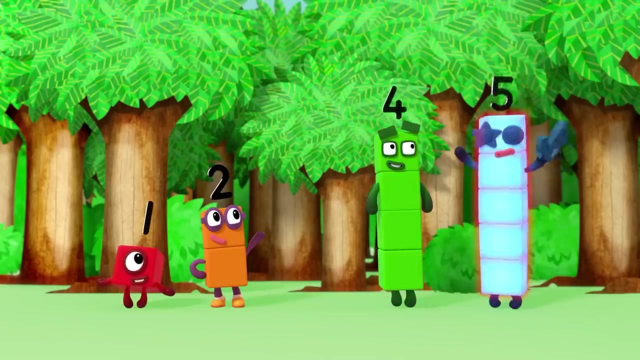 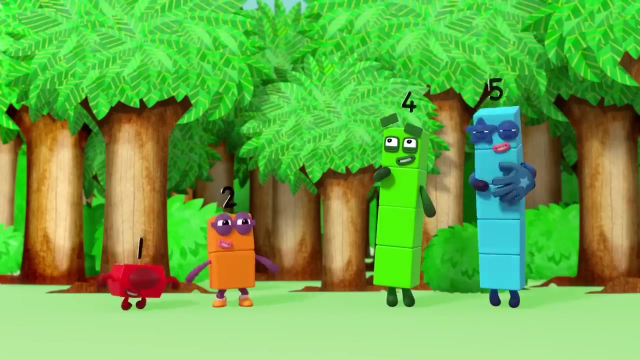 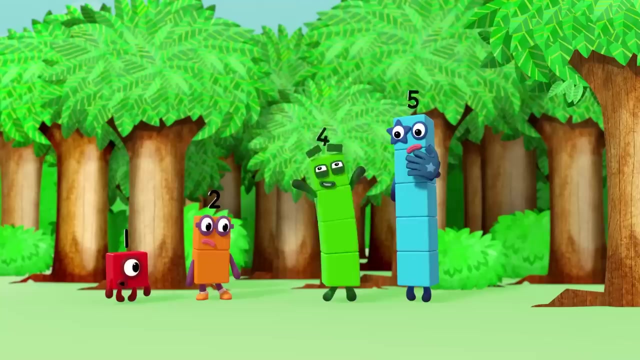 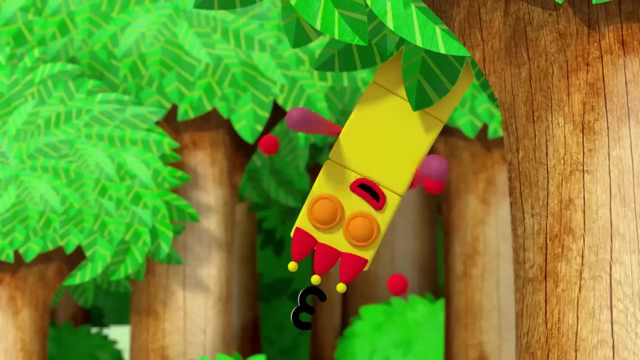 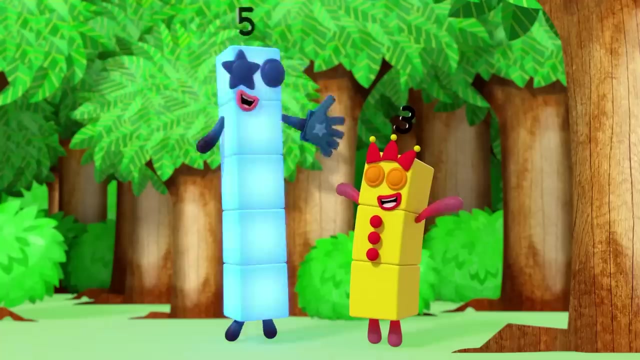 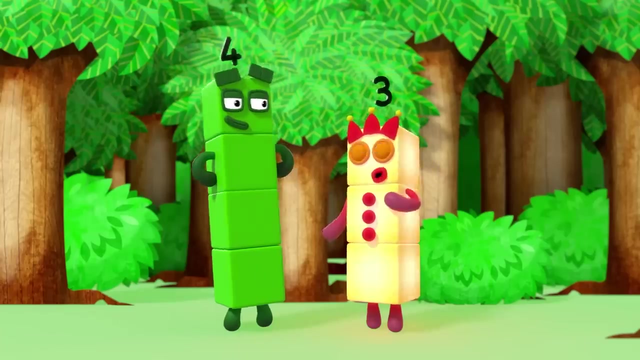 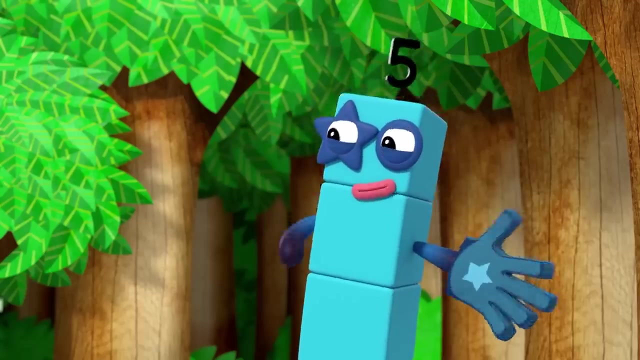 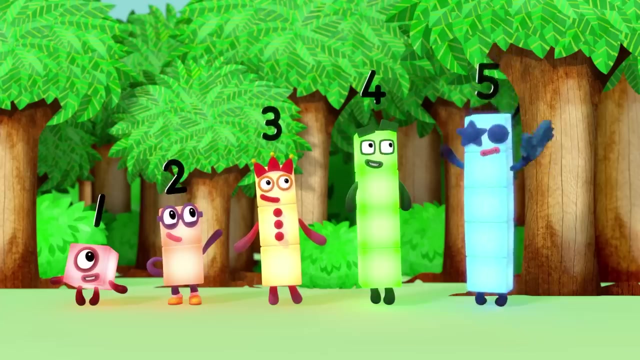 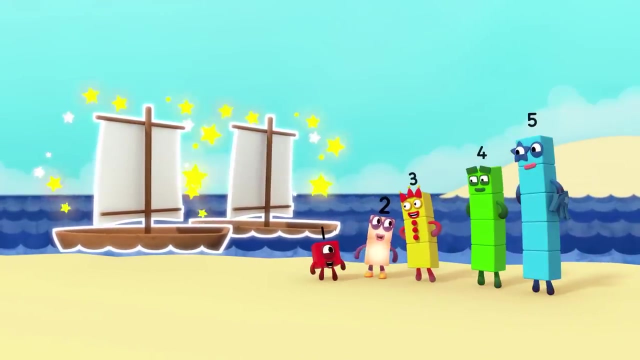 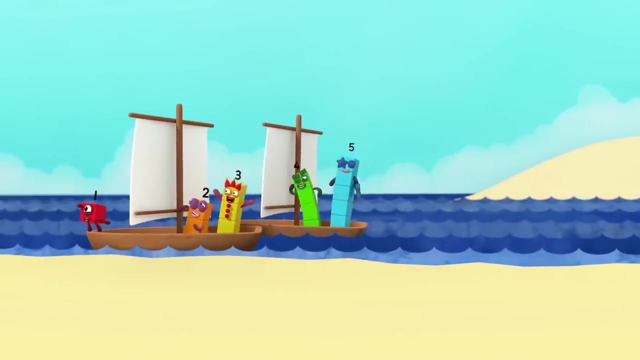 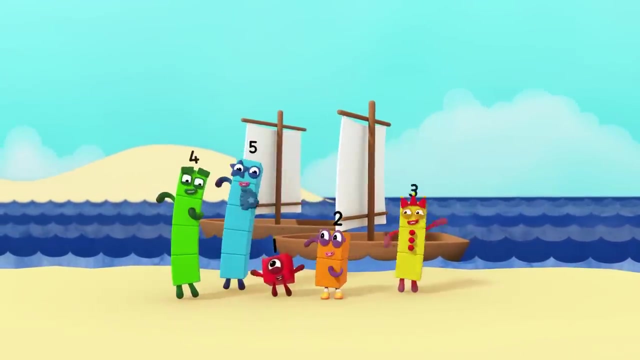 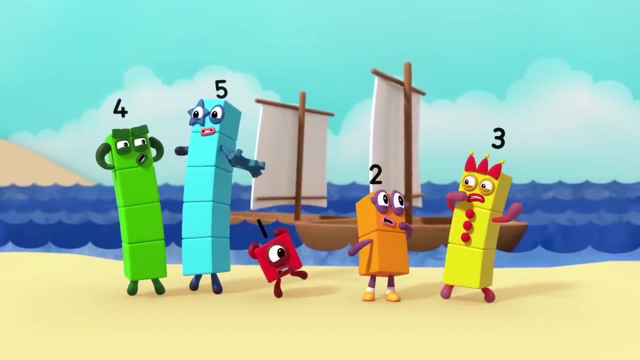 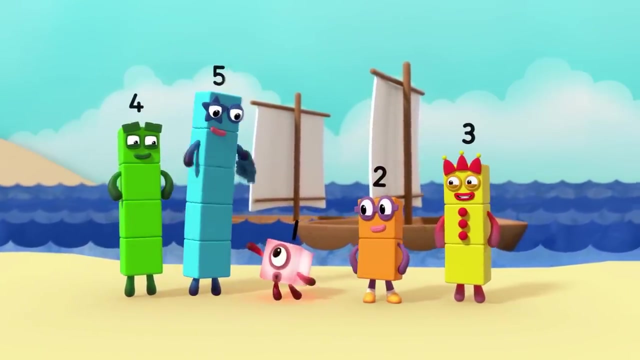 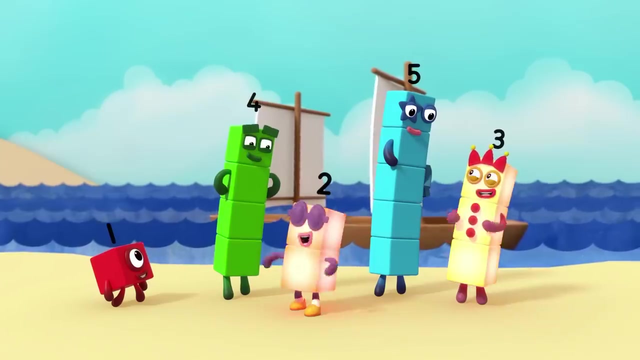 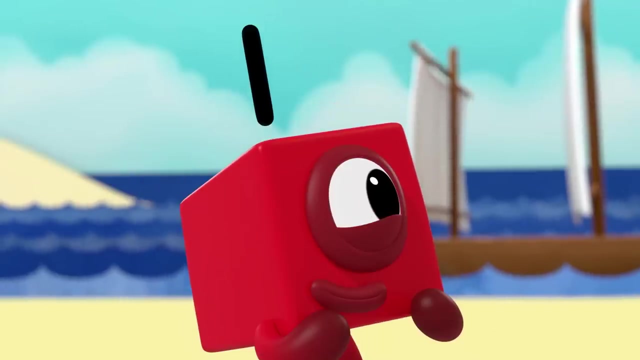 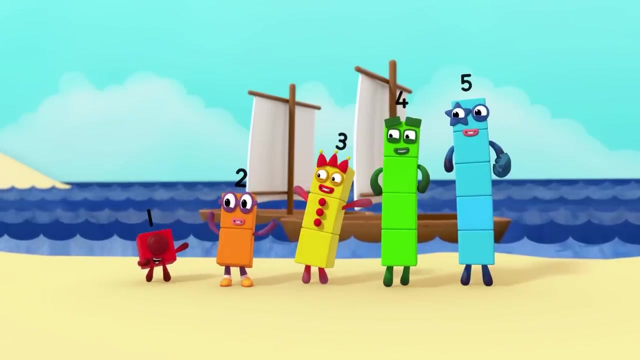 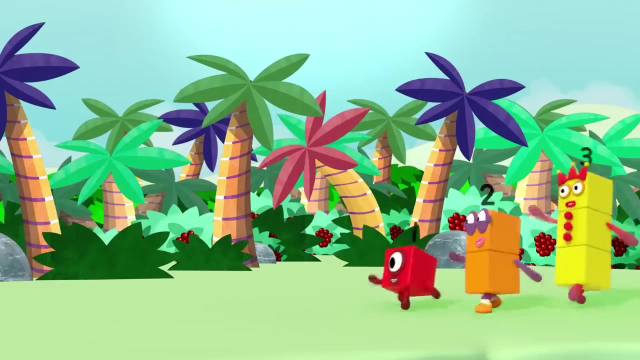 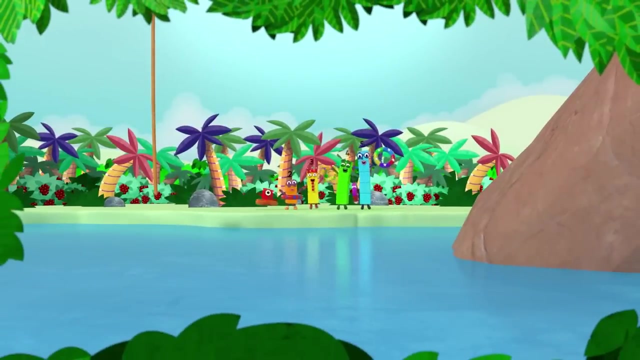 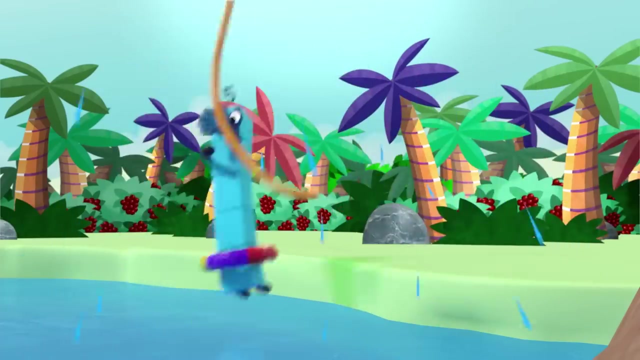 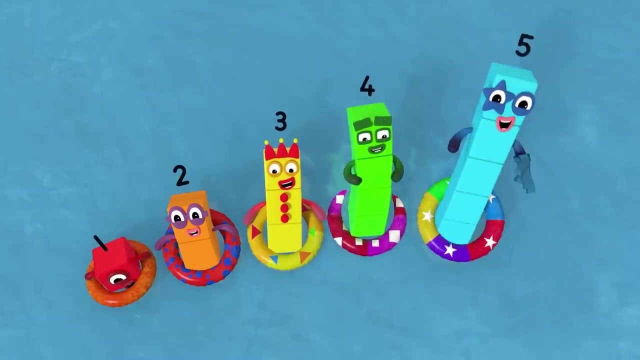 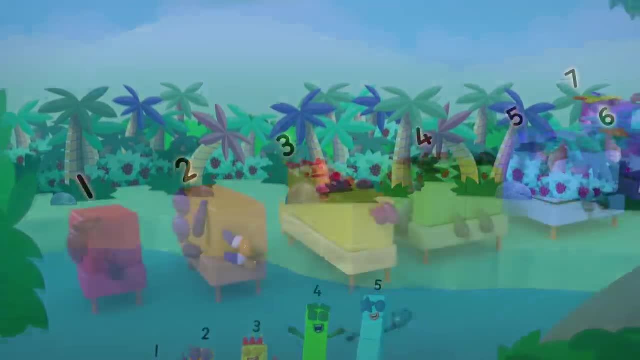 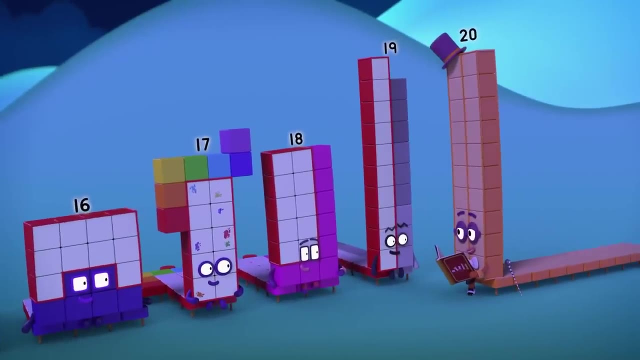 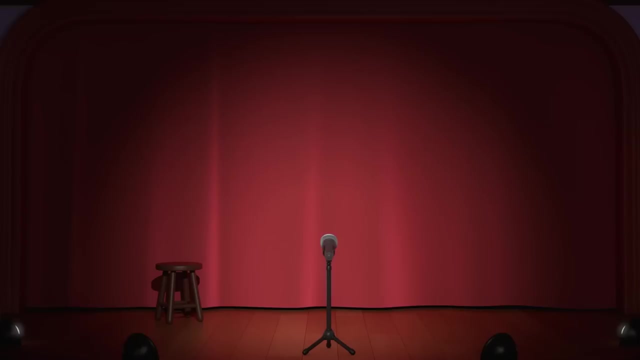 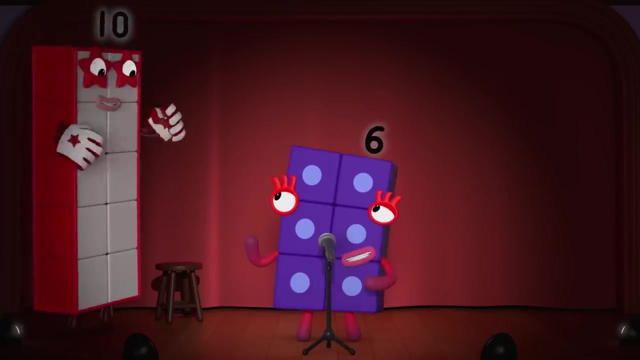 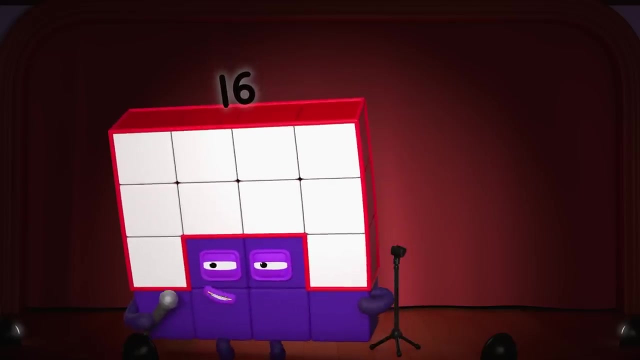 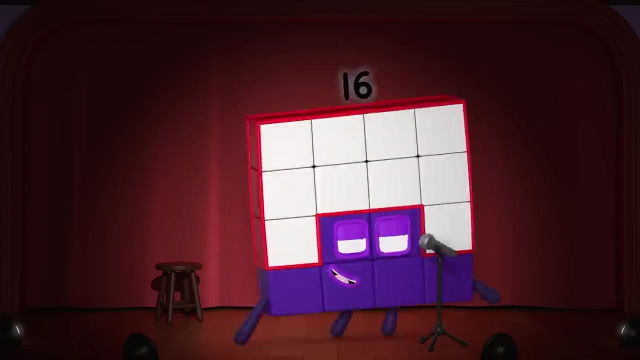 Subtitles by SteamTeamExtra. Um hi Ten, I'm 16.. Right here, I'm 16!. Let's get this party started. It's nice to be here And here and here and here. Oh, look at that. 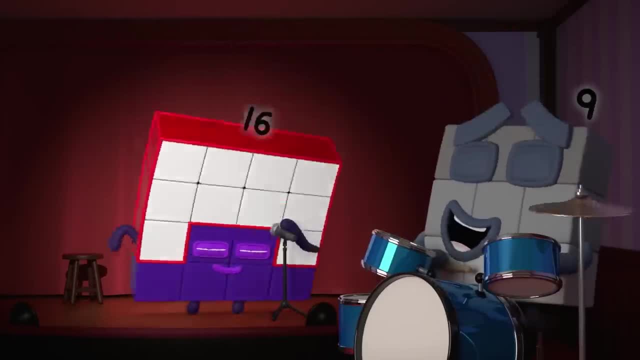 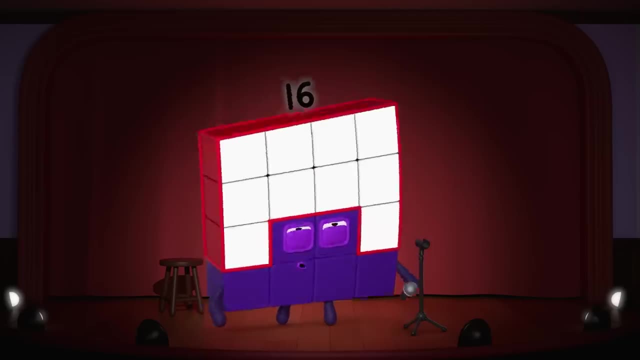 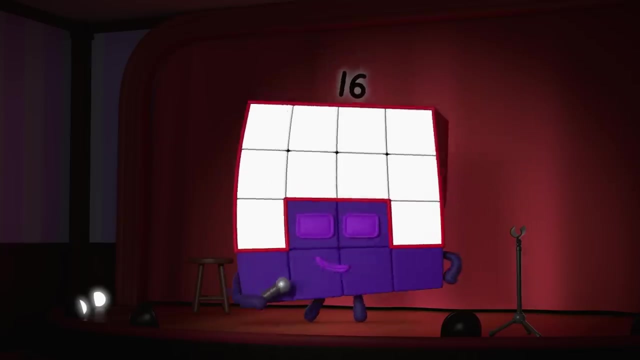 I'm square turning round. Hey, you know what Nine's favourite story is? Goldilocks and the Three Squares Squares. And if you're after a square deal, here I am. I'm a square Made of squares. 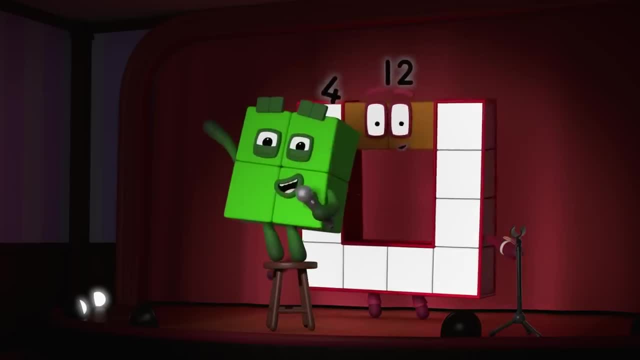 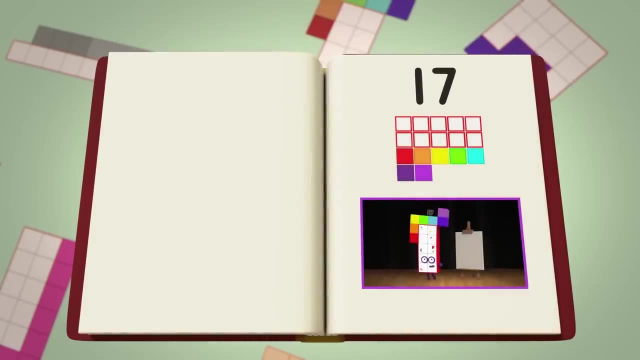 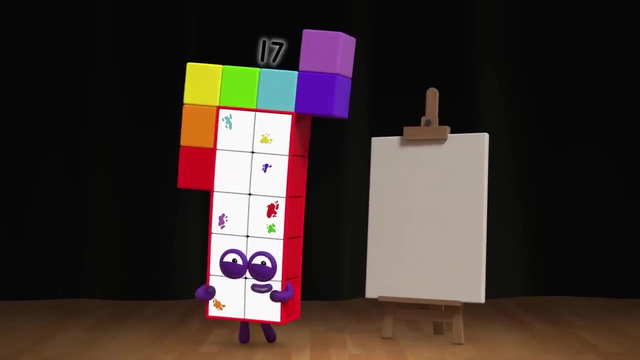 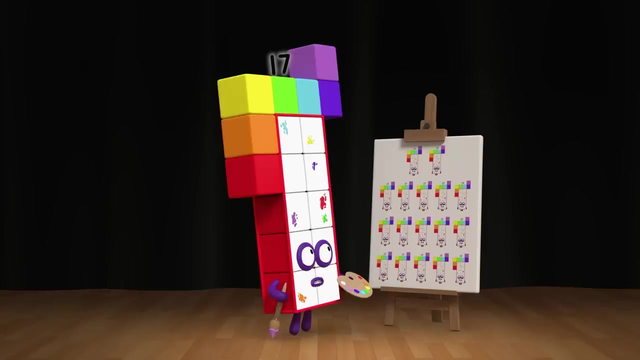 With a A square in the middle, Chapter 17.. Portrait of the Artist in His Prime Howdy 17. here Today, I'm going to show you how to paint a self-portrait. Here goes, Oh dearie me. 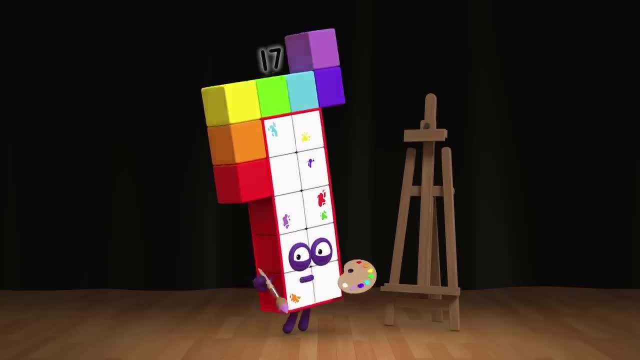 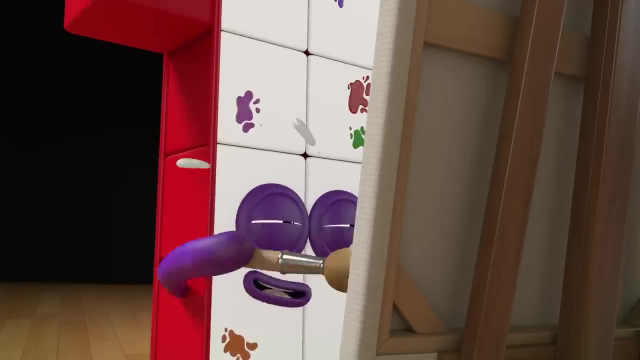 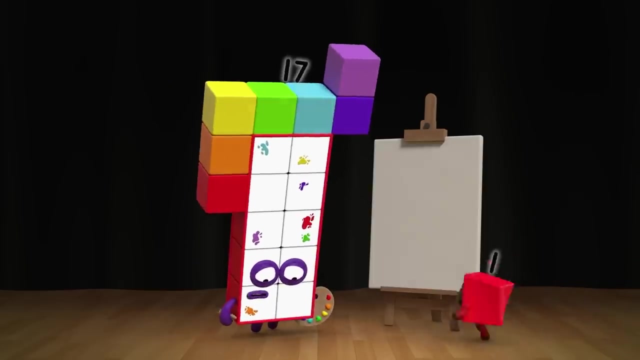 That's 17 self-portraits. Let's try again. I'm 10 and 7! So if I paint 10 and then 7.. Oh, 17 of each. Oh, I'm never going to get this right. 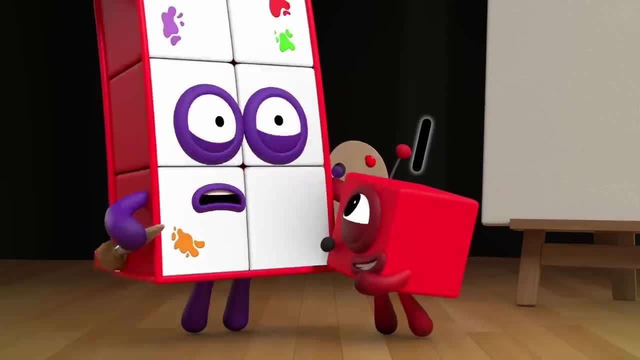 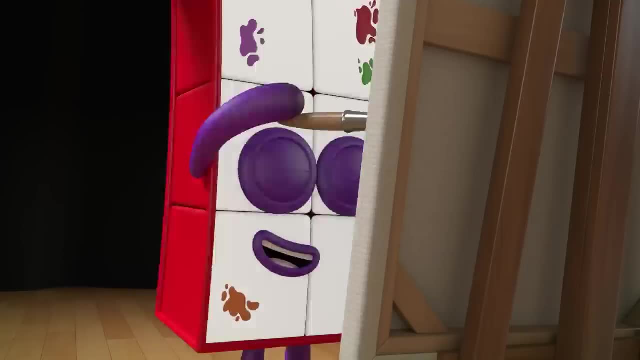 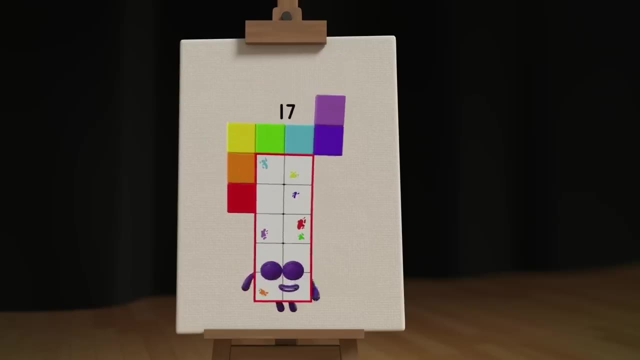 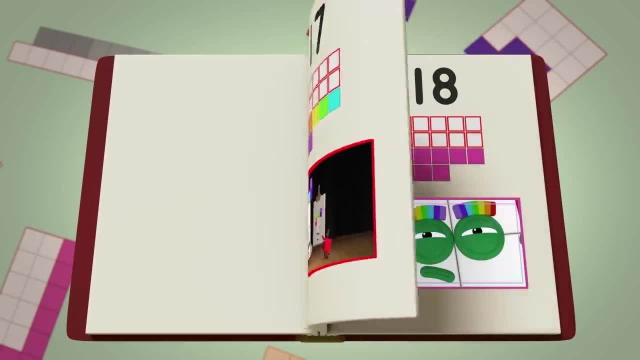 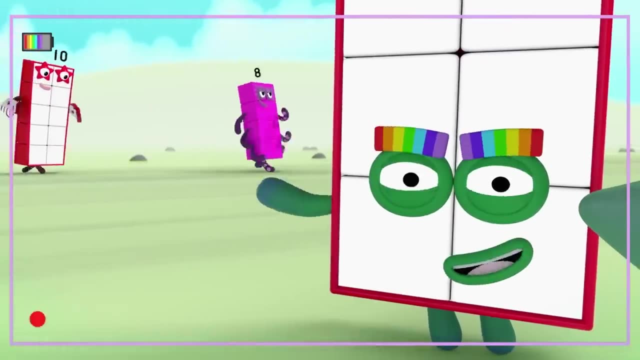 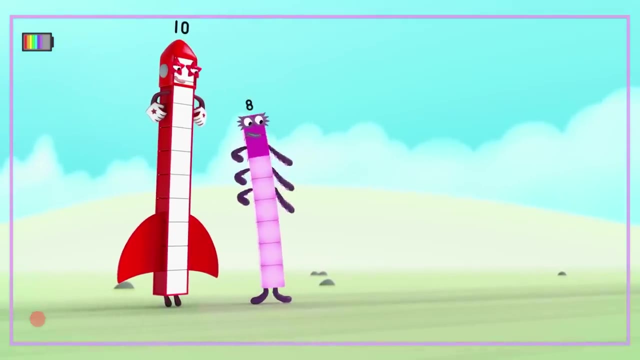 Pretty as a picture, Chapter 18.. Full speed ahead. Xtreme 14 here Reporting live on a cool attempt to be the fastest number ever. Rocket 10, ready to fire 2-4-6-8!. Super speedy. 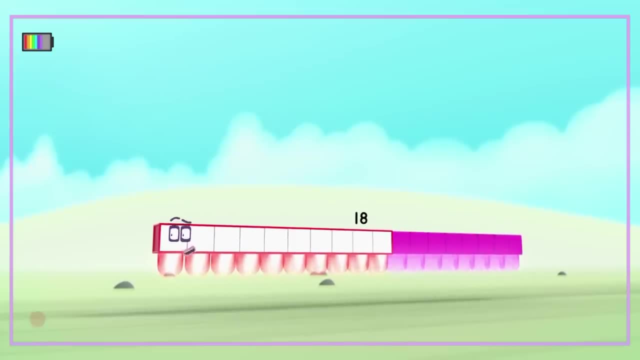 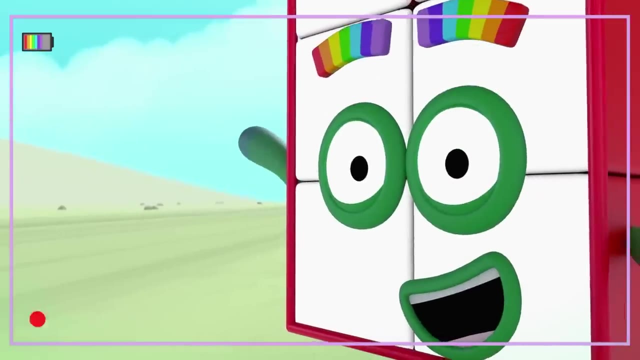 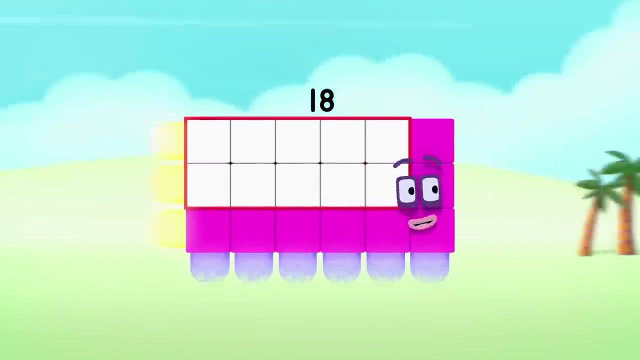 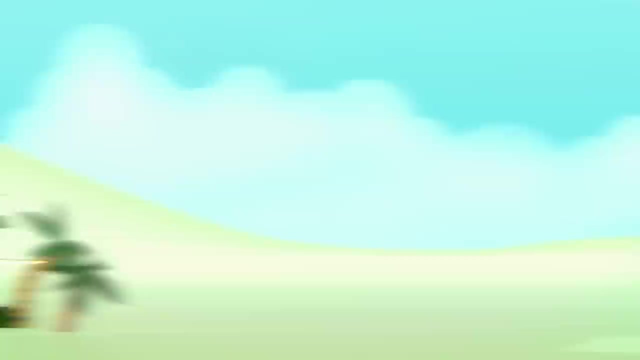 Don't be late. Then Somebody say speed 18!. Speed Machine, One ray and away. Wanna see me go faster? Two rays and away. Three rays and away. Six rays and away. Nine rays and away: Super Sonic. 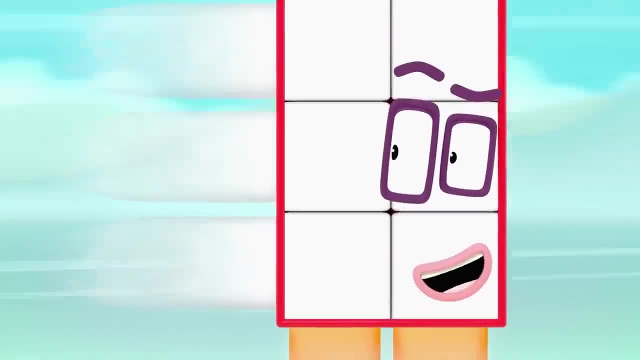 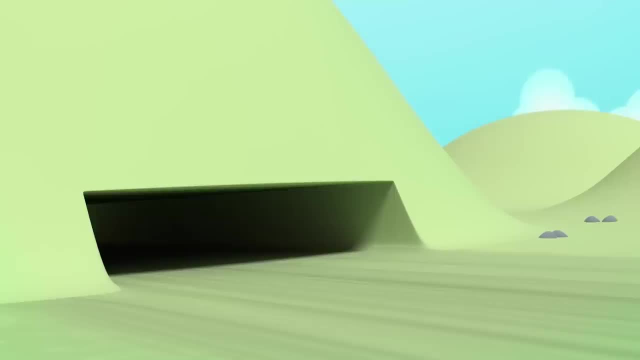 18!, 18!, Good call confidants. Three 18! Rays and away Go dude, Look out Tunnel. Uh-oh, Ah, Now that was a speedy escape. Phew, Chapter 19.. 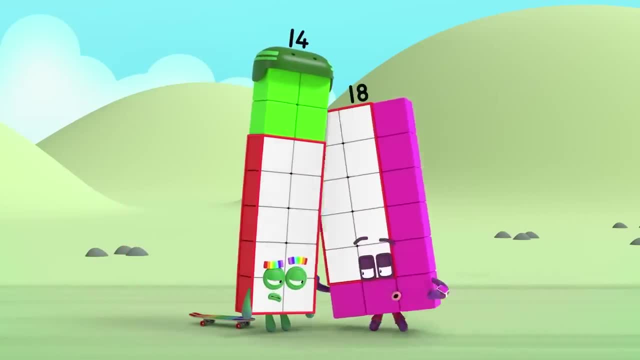 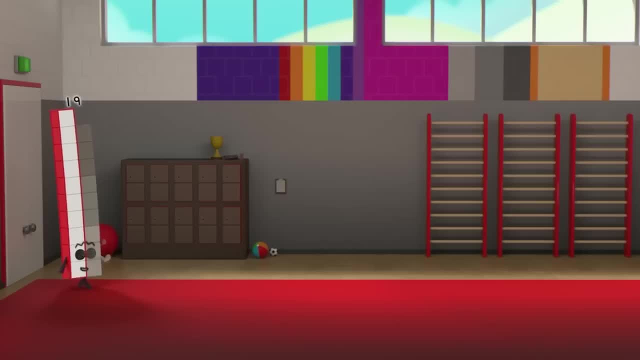 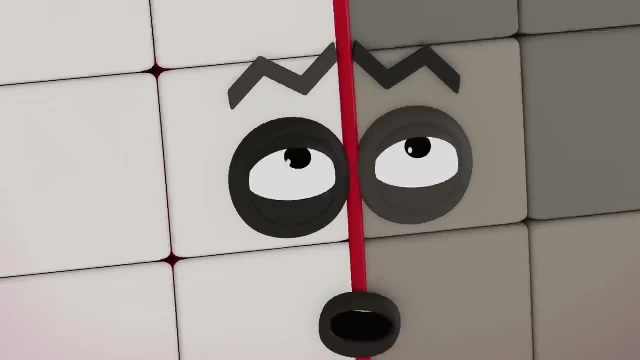 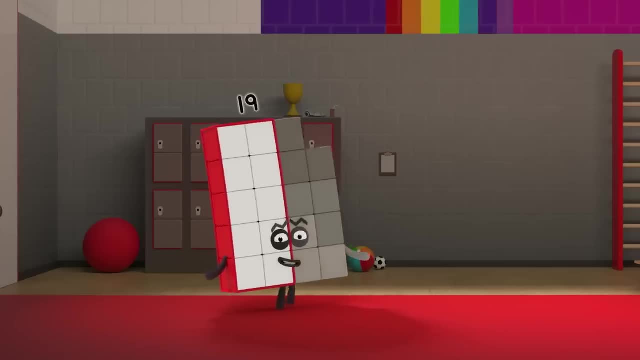 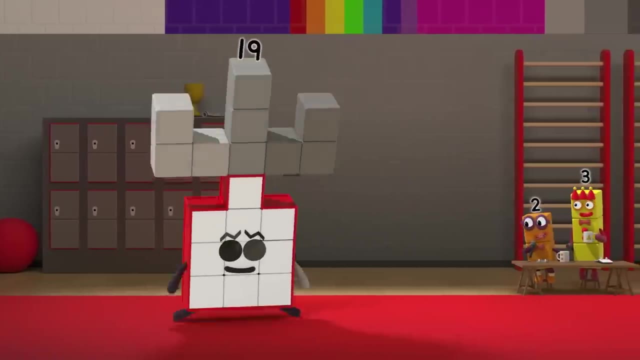 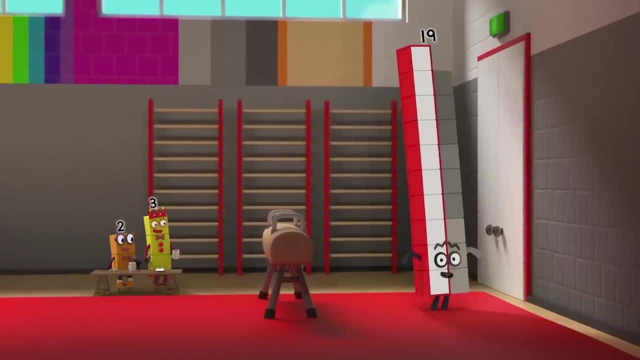 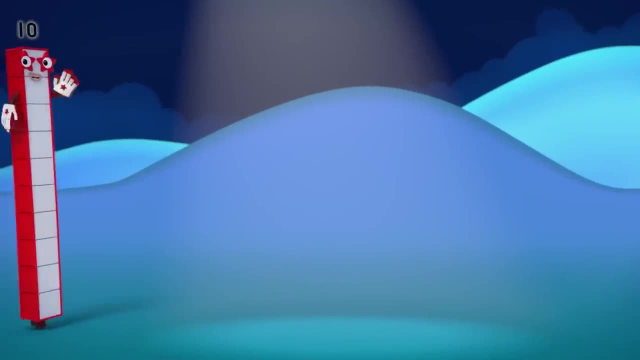 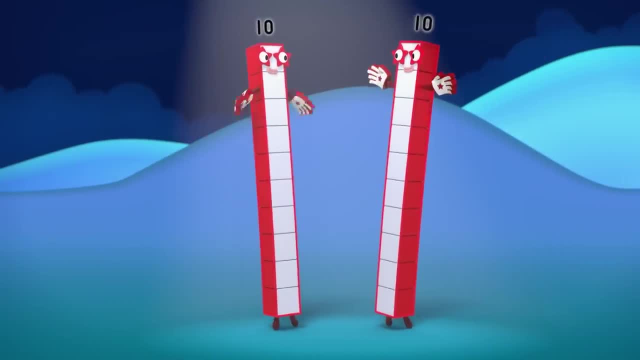 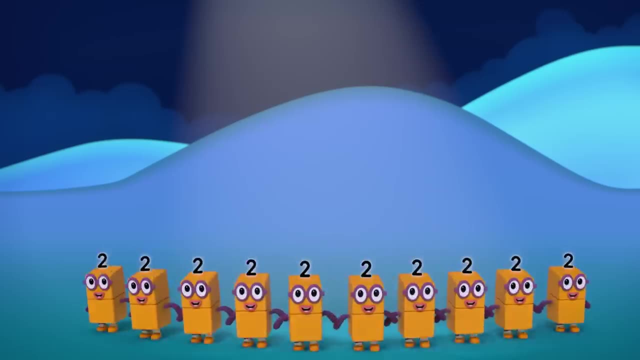 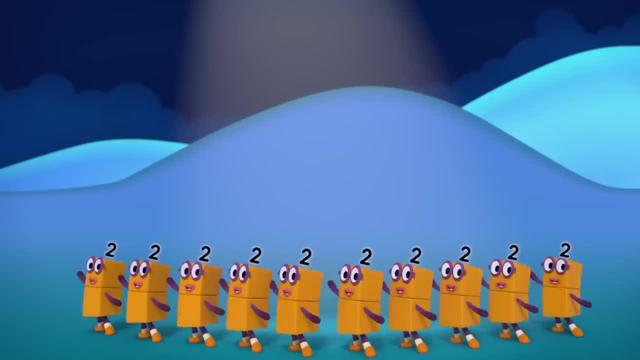 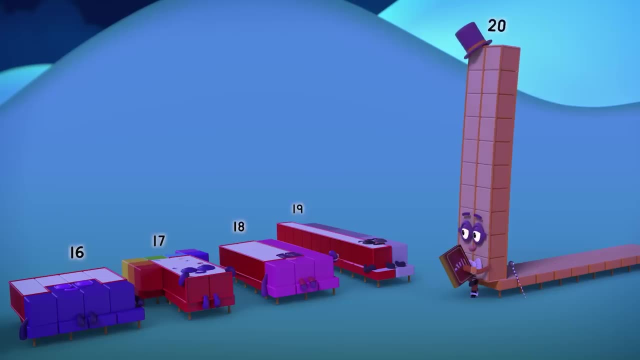 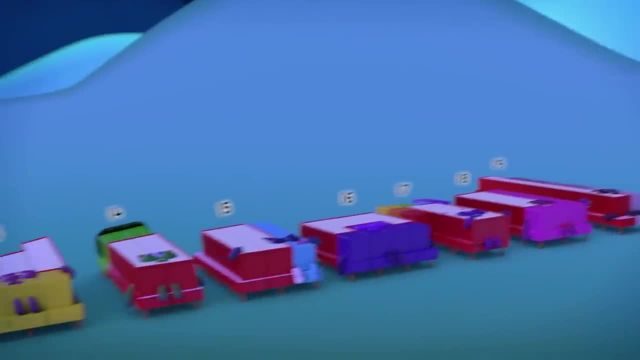 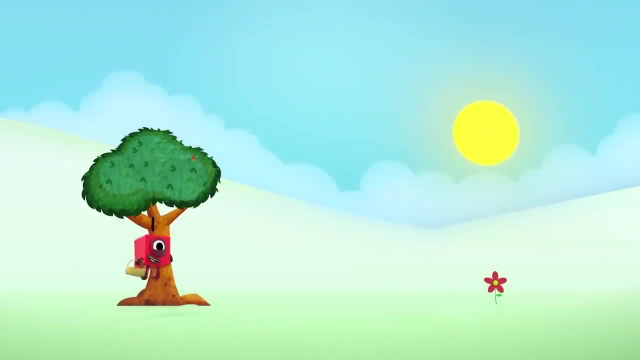 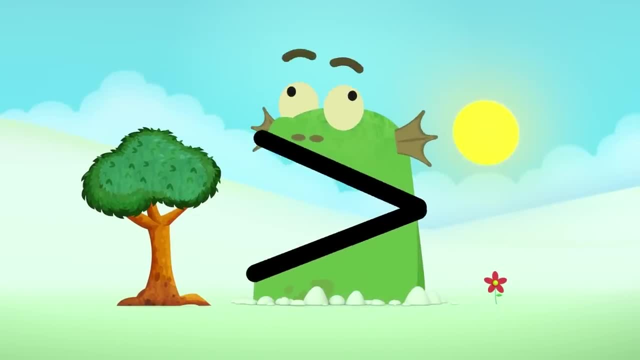 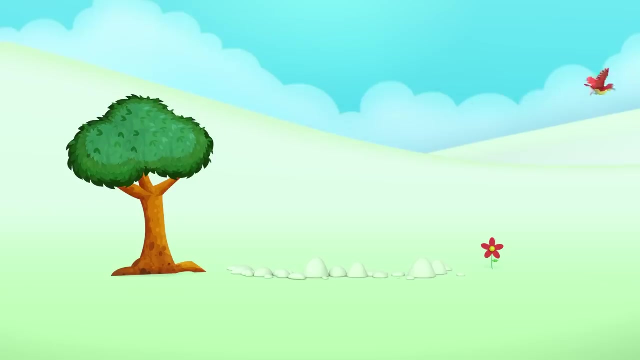 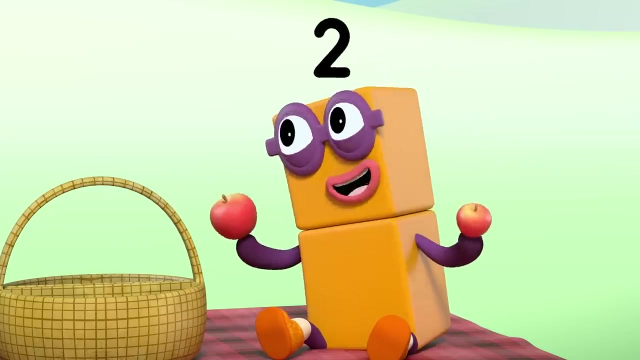 I'm 19! MeBlockzilla. Me like big things. Which is bigger? Tree is bigger than flower. Me like tree. Nice to meet you, tree. Will you play with me? This apple is bigger than this one And you're bigger than me. 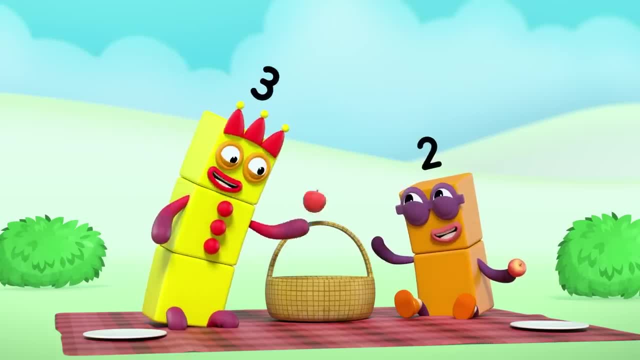 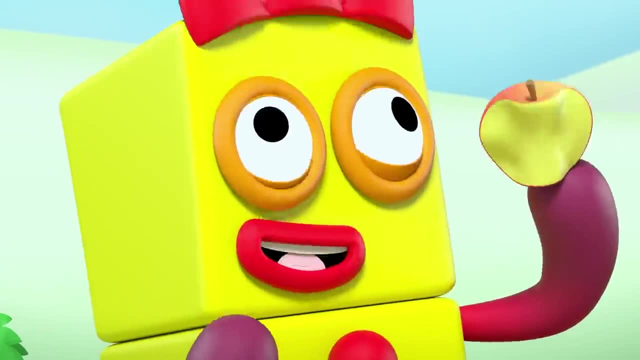 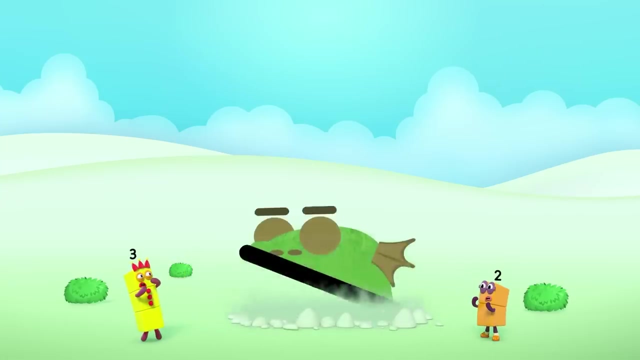 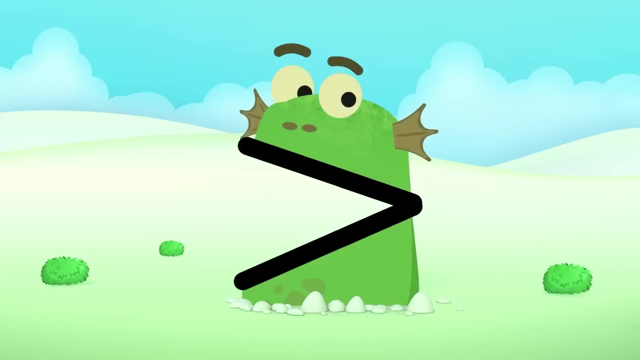 So you have it three. Thank you two. I like apples, I like to munch them And crunch them And gobble them up. Me Blockzilla Three has more blocks than two. Three is greater than two. Greater means bigger, So me like three. Don't gobble me up. 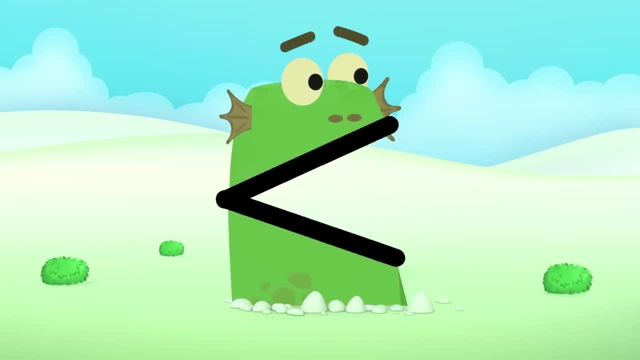 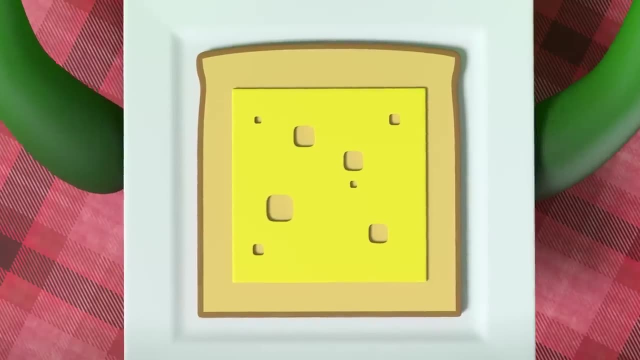 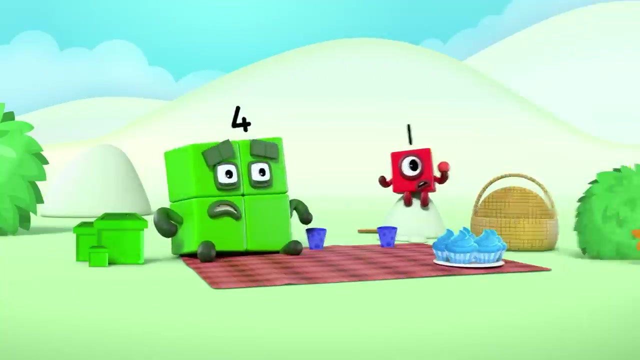 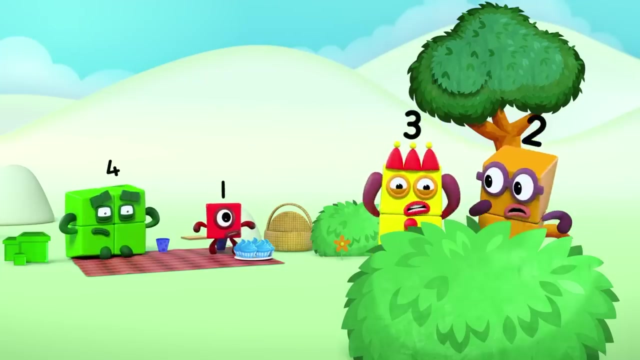 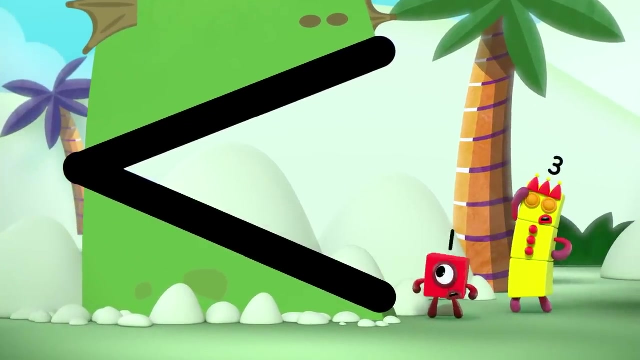 Me, don't eat you, silly Me, like you. Oi, Oi, I like square cheese. I like it in my tummy. There's a monster. It wants to munch us, crunch us, Gobble us up. Run hide. Look a cave We can hide in there. 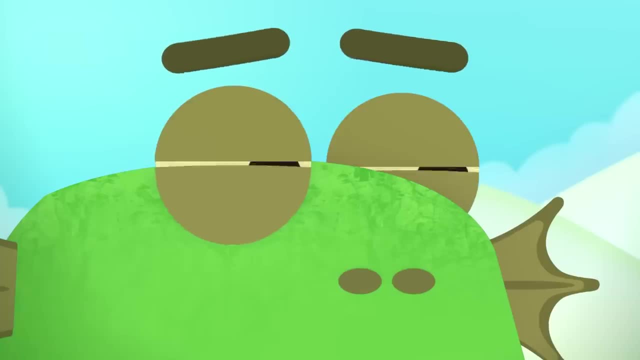 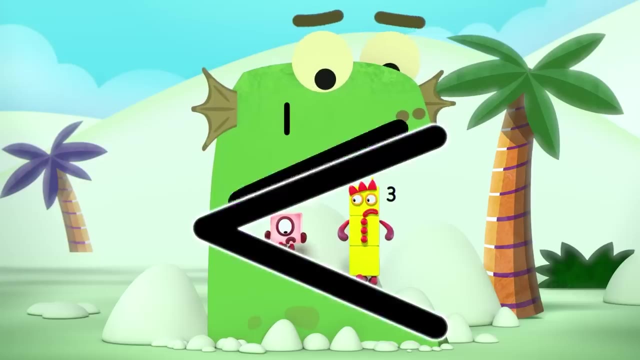 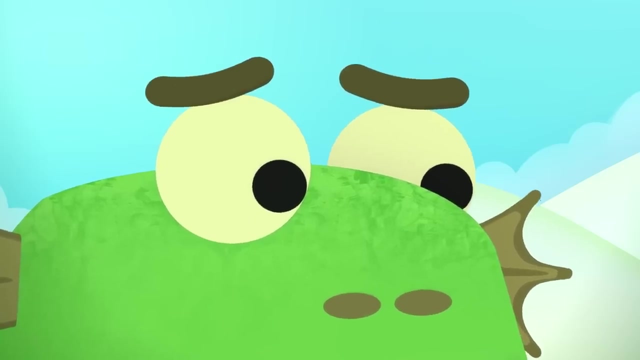 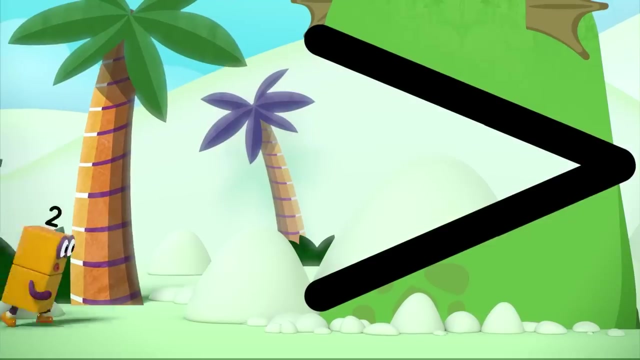 You go first. one: You're smaller than me. We should be safe in here. One is less than three. Me like bigger numbers, So me like three. Me want to meet you, Not eat you. Where can we hide? Look a cave, You go ahead. two: 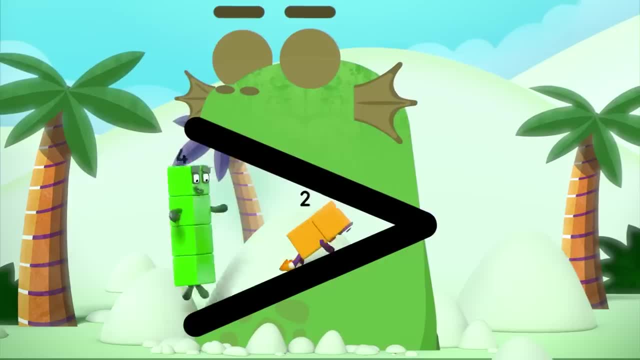 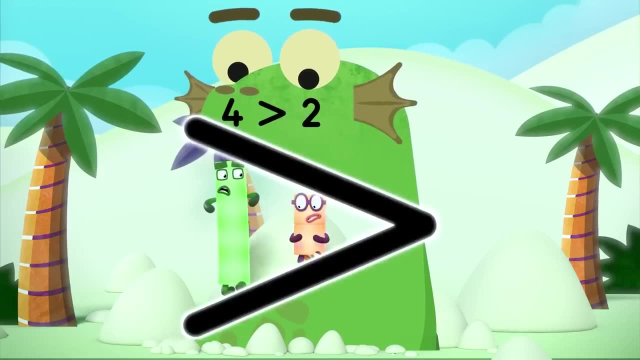 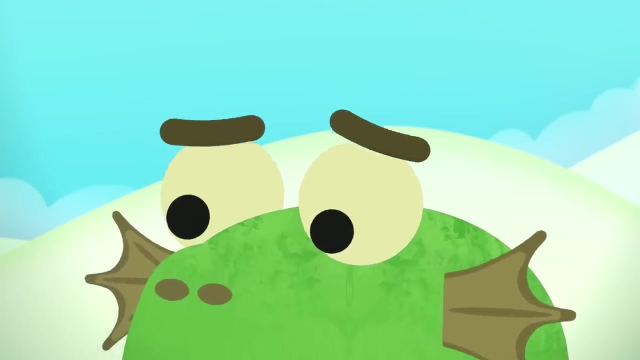 I'm bigger than you. We should be safe in here. Four is greater than two, Though me like four- Excuse me for the silence- Like I like square cheese In my tummy. Ahhhhh, Ooooo, Noooo, Silly, Oh, dear. Sounds as if we need a plan. 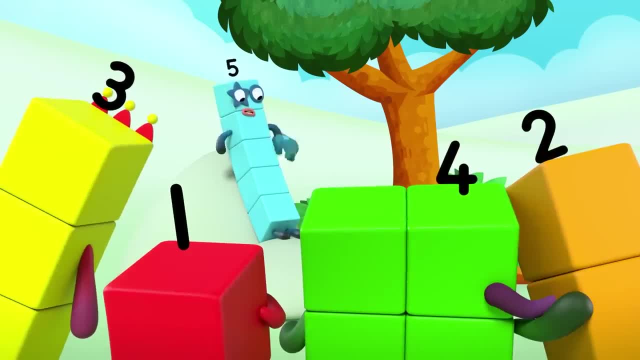 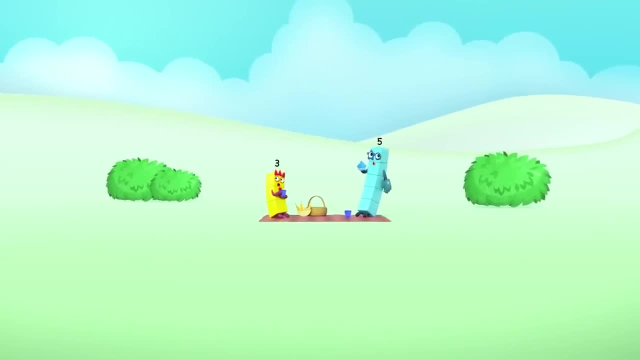 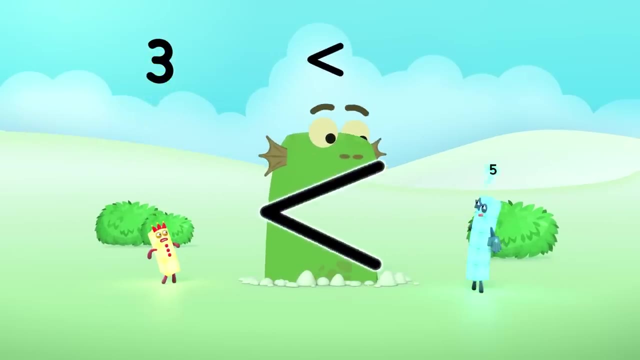 And I think: well, what if I, I, I, I would be the loudest. Three is less than five. Me like five Gah. Me mean five is greater than three. Me like five Gah, Three is less. 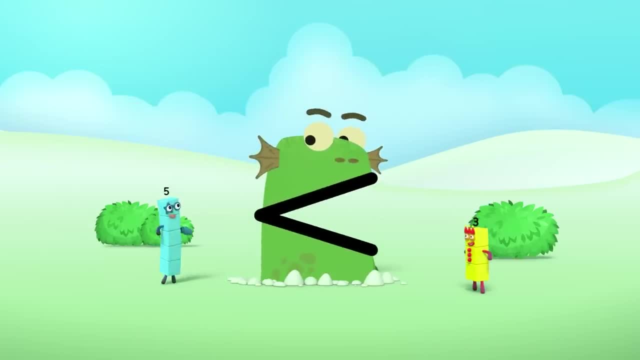 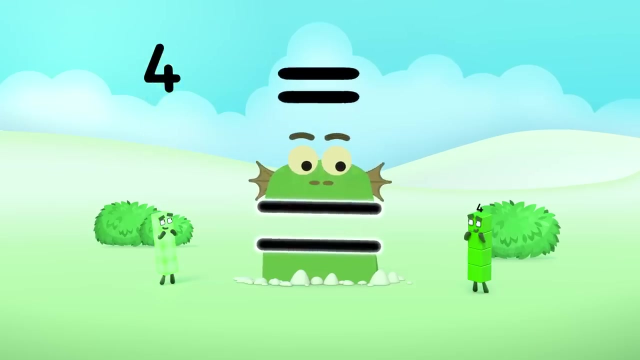 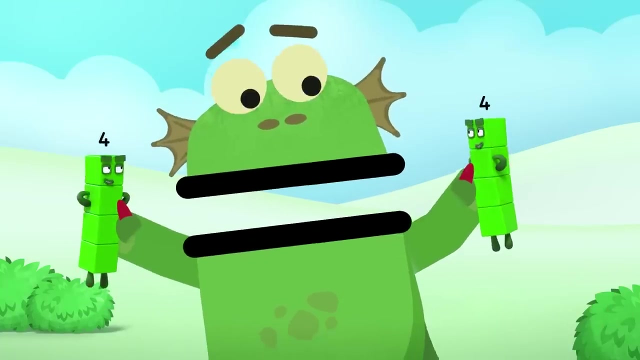 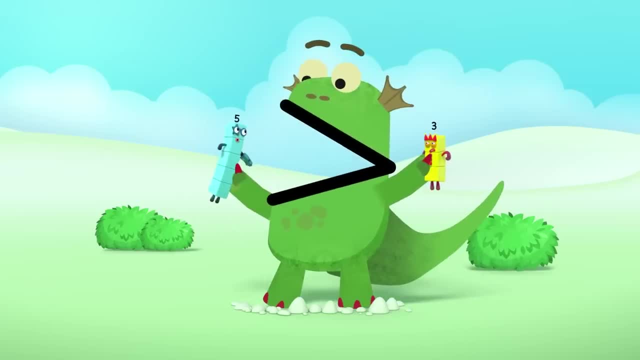 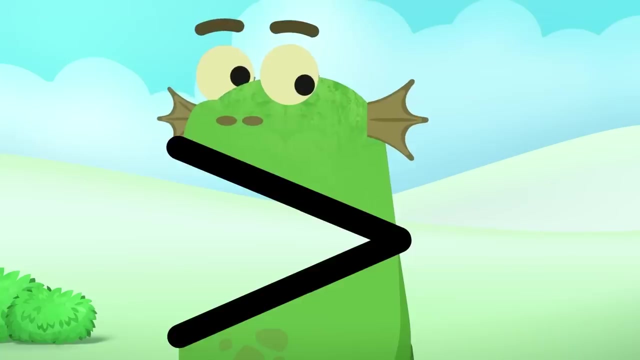 What me like to play with you? Play with us. Five is greater than three, so, Bloxzilla, play with five. What Whee Play with me? Play with me, Bloxzilla. play with number blocks. Three is less than three. 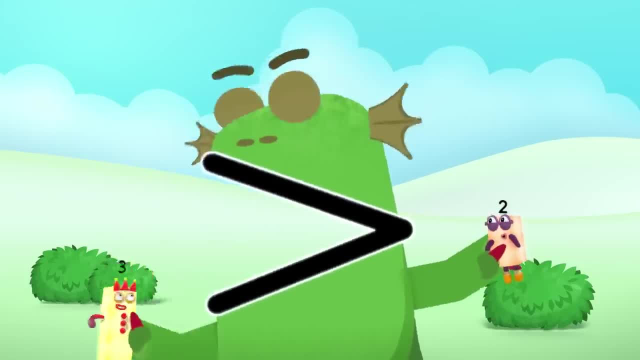 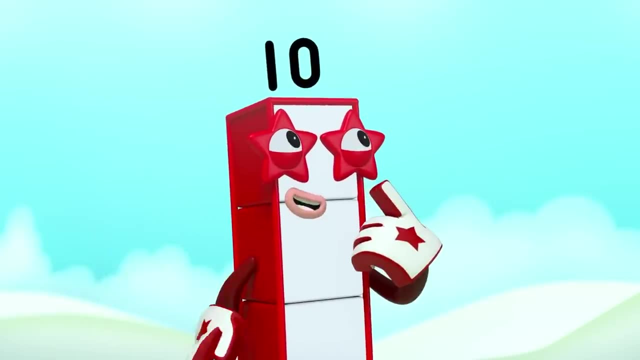 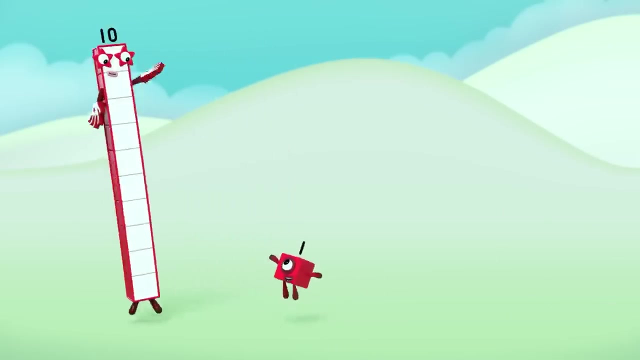 Four Three is greater than two. One, Hello one. What shall we play today? Oh Ooh, um hm. What was that? Who was that? A new number. block Ten plus one Equals 11!. 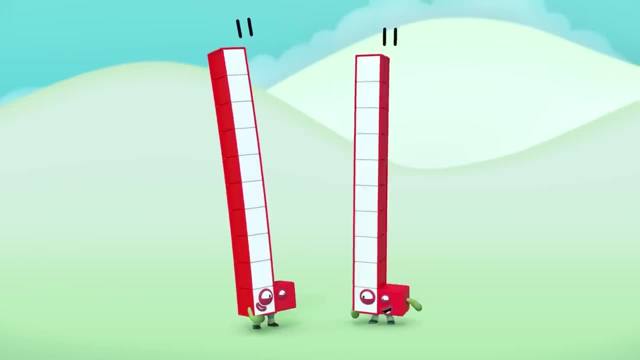 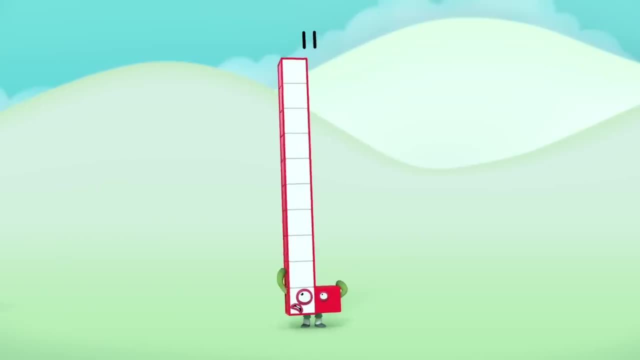 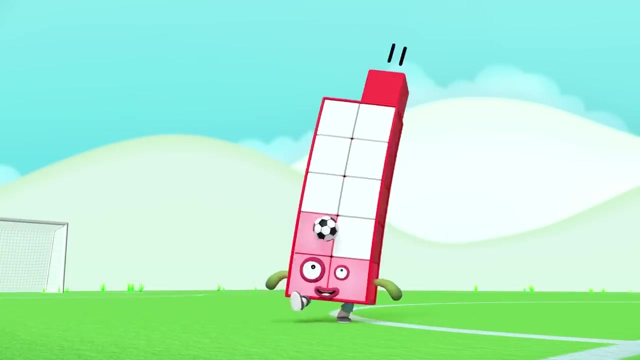 Hello, I'm 11.. So am I, And I'm 10 and 1.. That's better. Whoa: 1, 2, 3, 4,, 5, 6,, 7,, 8,, 9 and 10.. 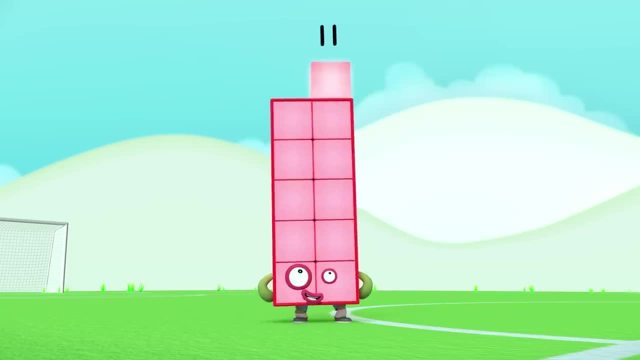 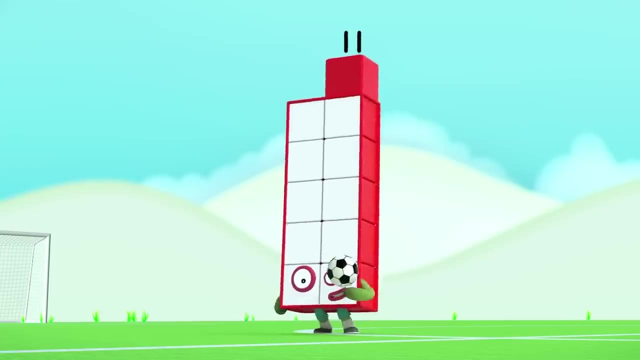 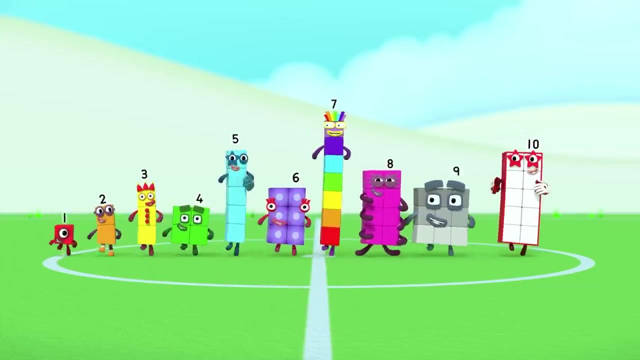 And one more is 11.. I am 11 and I love football. Wow, Let's play football, Hooray. 1,, 2,, 3,, 4,, 5,, 6,, 7,, 8,, 9 and 10.. 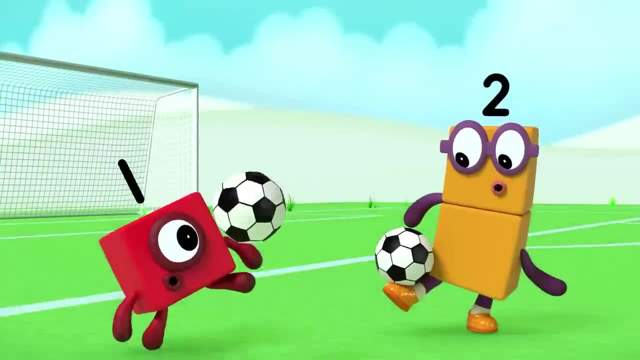 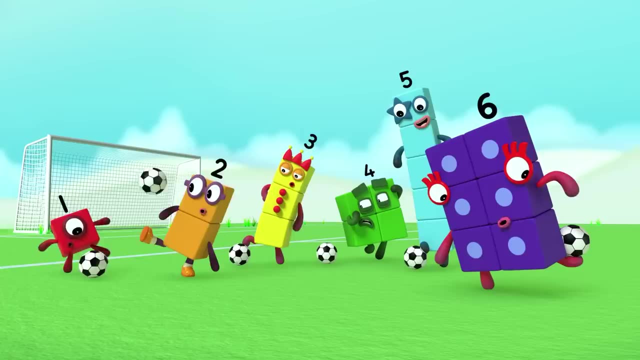 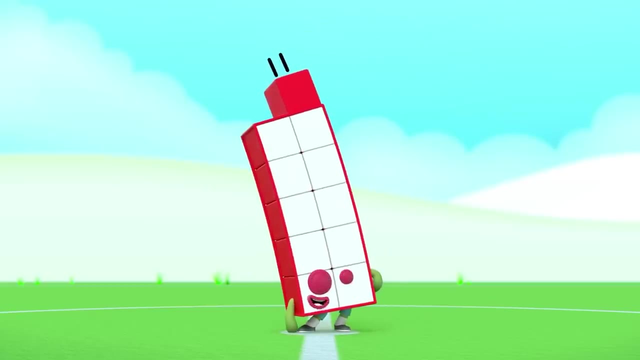 One more is 11.. We're on our way to victory. We're on a roll. We're ten on the pitch and one in goal. We will never be denied. We'll take it in our pride. We're 10 and 1, 10 and 1, 11 on our side. 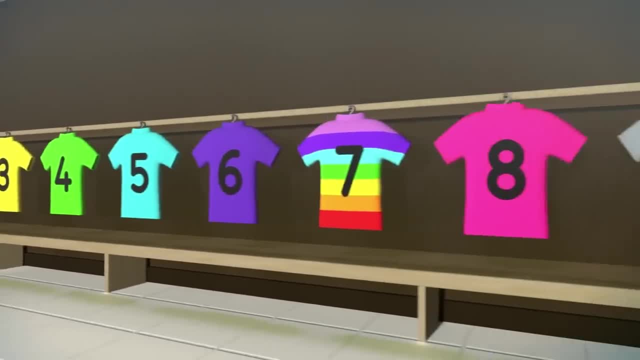 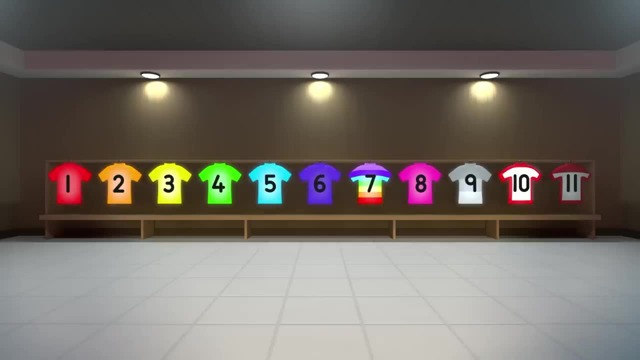 Football shirts. football shirts, One for every number. block Football shirts: 1,, 2,, 3,, 4,, 5,, 6,, 7,, 8,, 9 and 10.. And one more is 11.. 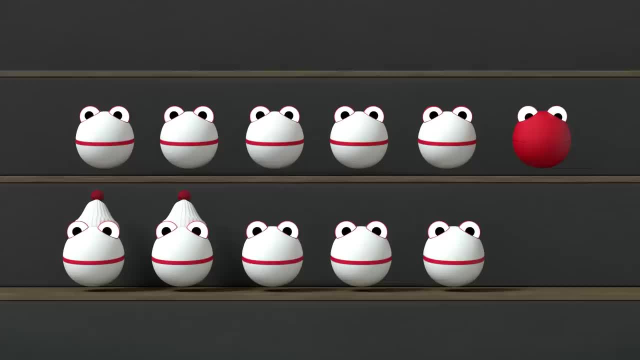 Hooray Bubble hats. bubble hats One for every number. block Bubble hats 1,, 2,, 3,, 4,, 5,, 6,, 7,, 8,, 9 and 10.. 1,, 2,, 3,, 4,, 5,, 6,, 7,, 8,, 9 and 10.. 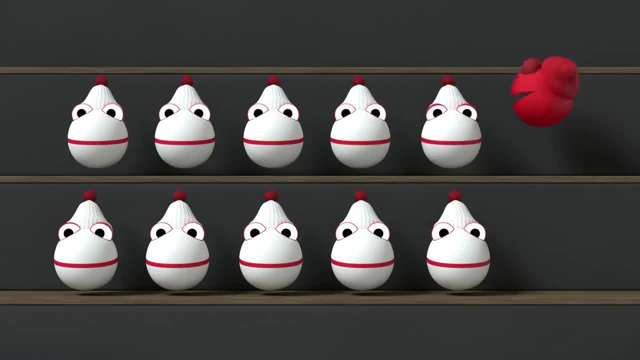 And one more is 11.. 1,, 2,, 3,, 4,, 5,, 6,, 7,, 8,, 9 and 10.. And one more is 11.. We're on our way to victory. We're on a roll. 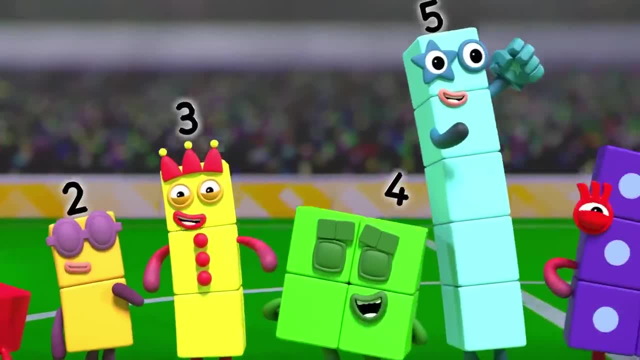 We're ten on the pitch and one in goal. We will never be denied. We'll take it in our pride. We're ten and one. ten and one, 11 on our side, 1, 10.. 1, 1.. 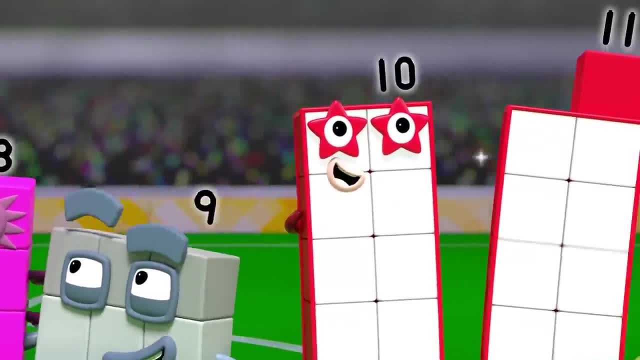 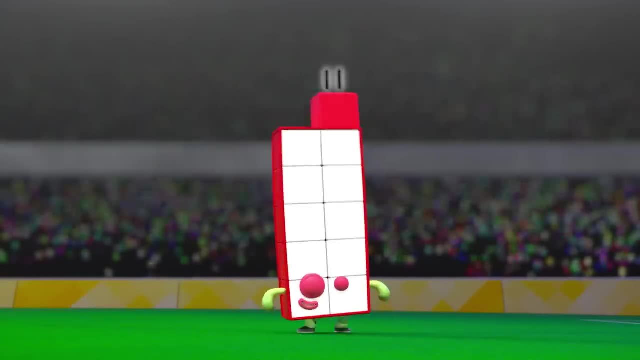 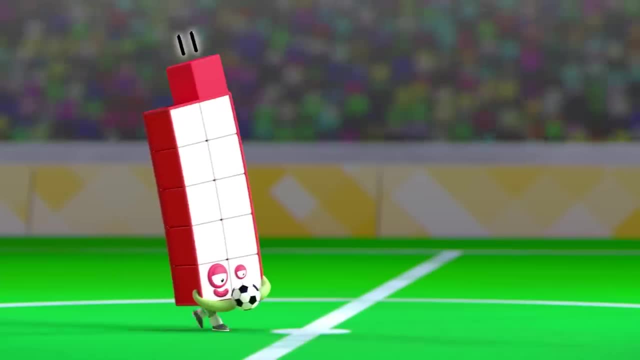 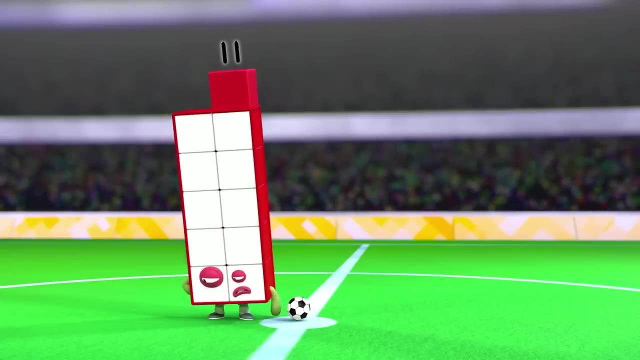 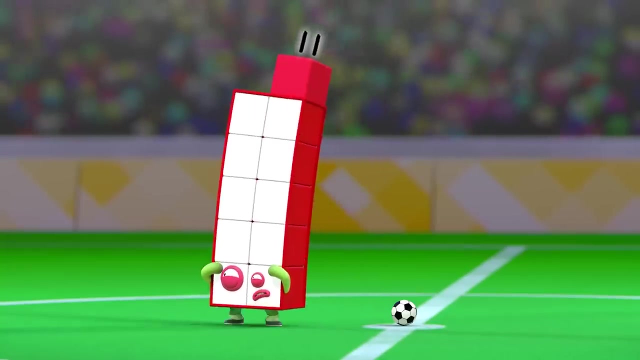 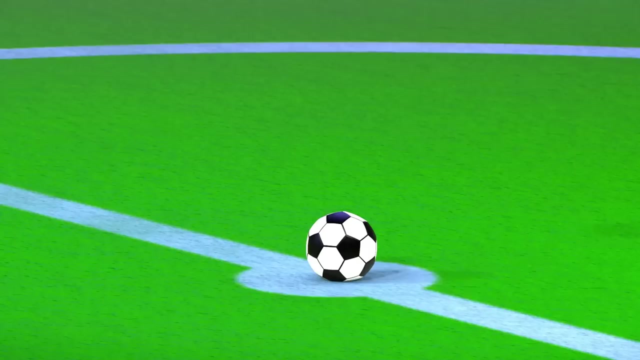 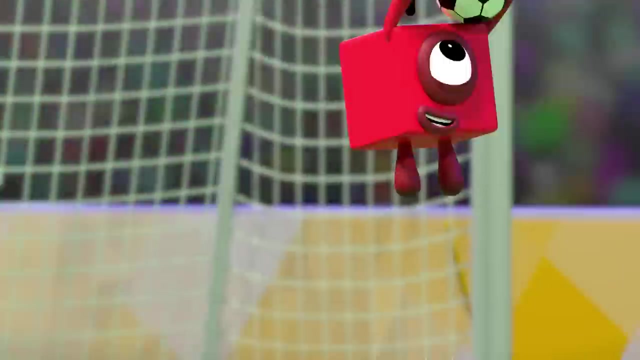 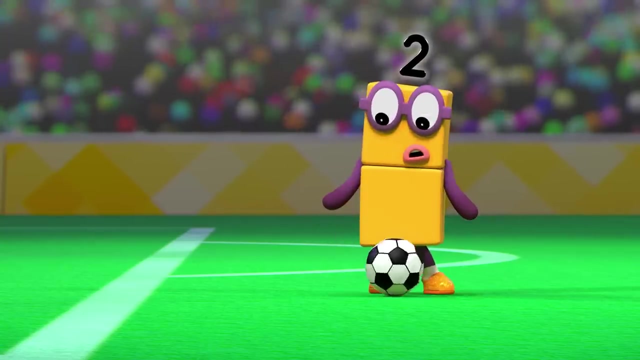 And one One, 12. chiaова, We win And the number balls have kicked off. It goes high towards the goal And, saved by one, Take a bow, one. One throws it down to two. Who passes it? 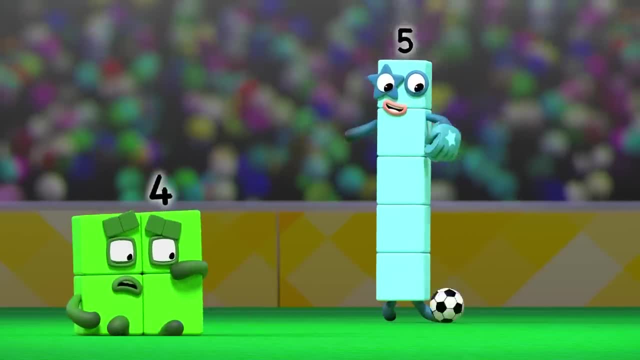 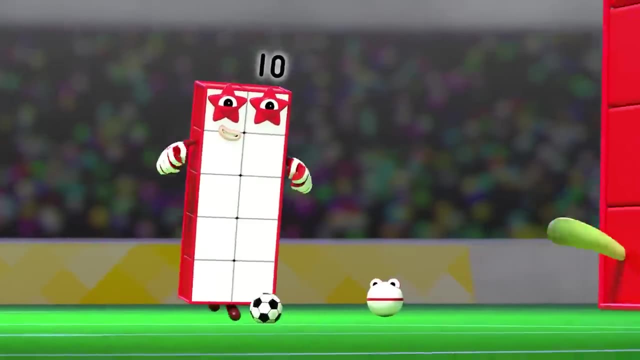 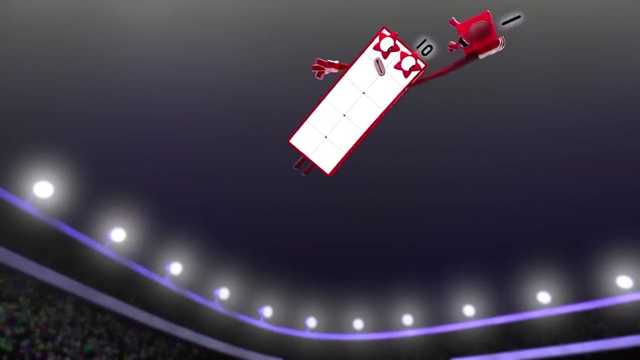 That's right to three, Four, Five, Six, Seven, Eight, Nine And ten. Now pass it to eleven. Ten passes, Eleven leaps for the header and, oh my splits into ten and one to reach the ball. 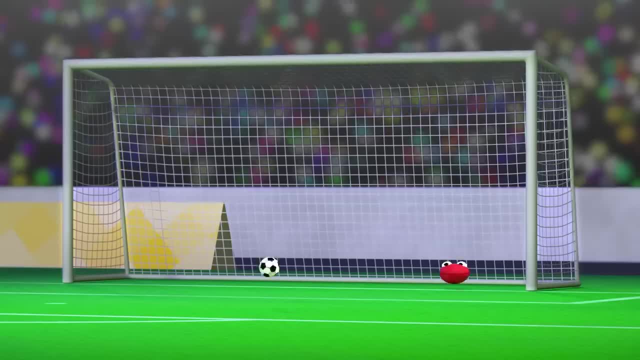 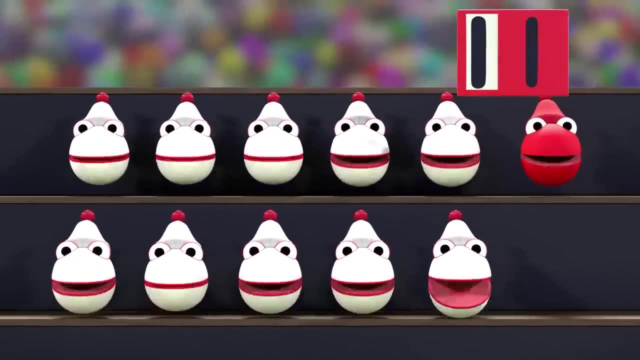 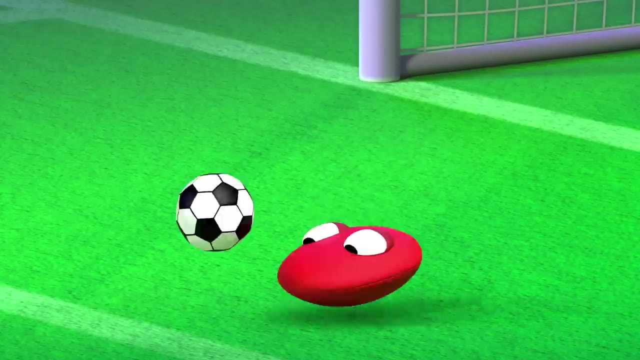 Incredible, And it's a save. What a save. Cut it up to eleven. You're louder than the rest. Ten and one. Ten and one, Seven is the best Number blob passes to number blob. Who finds number blob And a lovely header there to number blob. 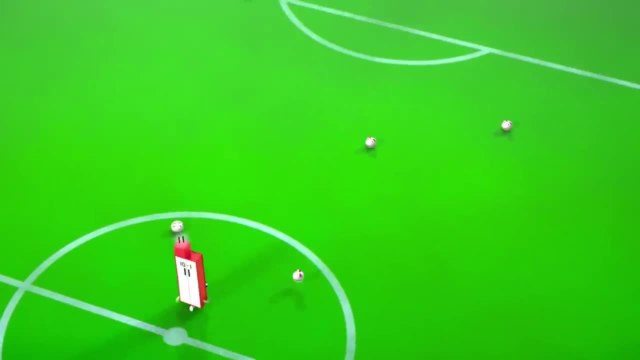 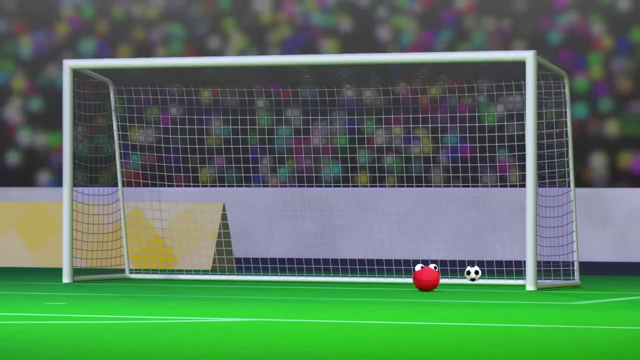 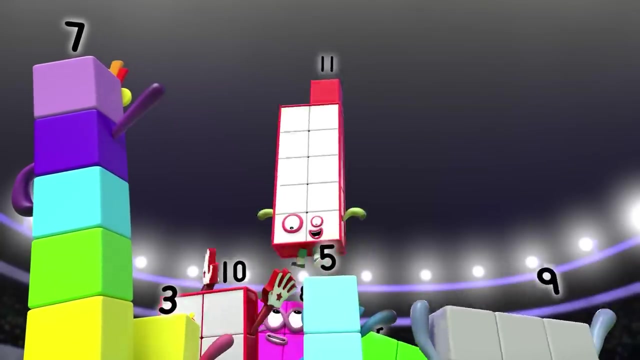 Eleven, Who heads it to eleven? And it's eleven, Eleven, Eleven, Eleven, Whoa Yeah, Goal, Goal. We're on our way to victory. We're on a roll With ten on the pitch and one in goal. 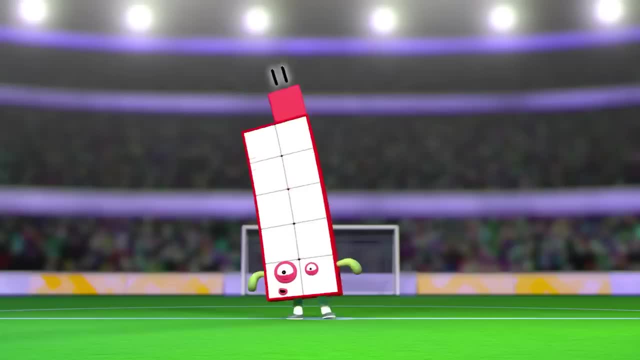 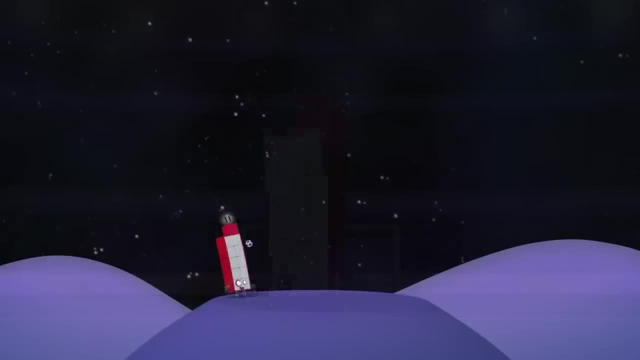 We will never be denied. We'll take it in our side, With ten and one, Ten and one Eleven on our side, Ten and one, Ten and one, Ten and one Eleven on our side, When worlds of wonder want exploring. 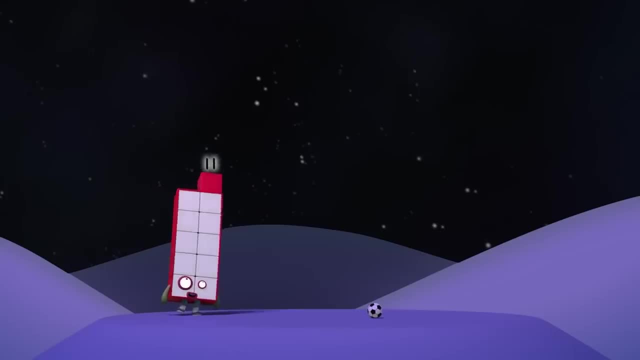 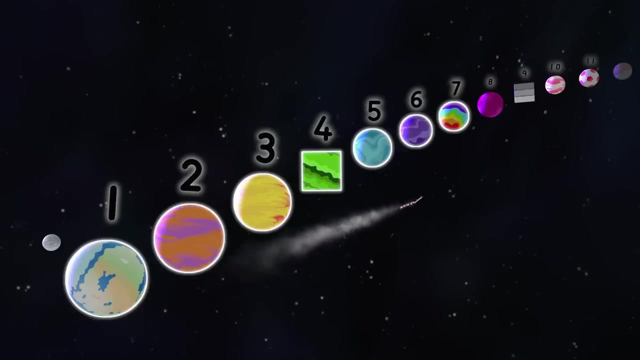 flights of fancy set you soaring Once you find your inner rocket. nothing in this world can stop it. Oh yeah, Eleven splits and ten and one blast off beneath the setting sun. One, two, three, four, five, six, seven, eight, nine, ten. 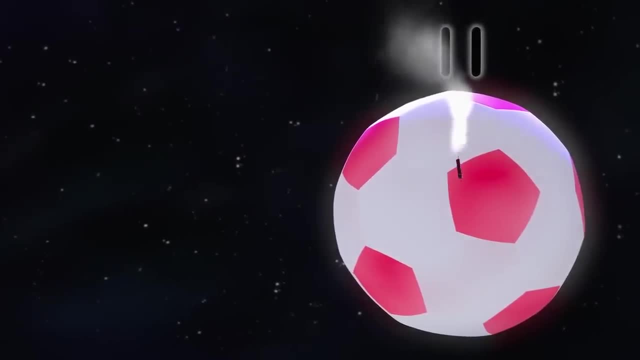 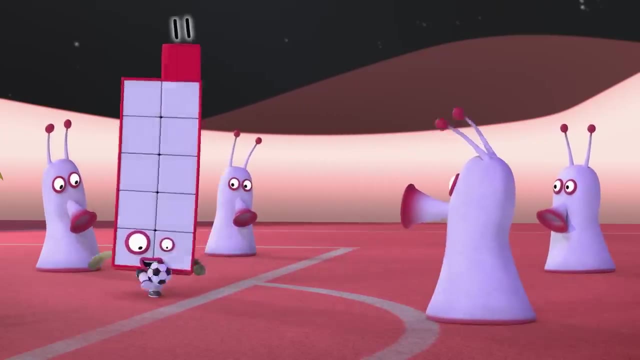 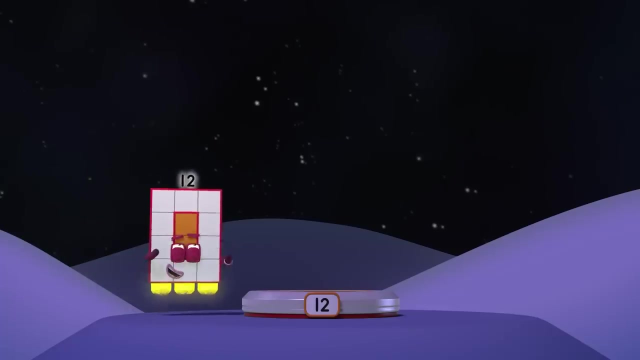 And one more race. Planet eleven, One plus ten has come to play A football match the alien way, And now they've seen the rocket blast. Others want to follow fast. Twelve is next to want to fly, So ten and two ascend the sky. 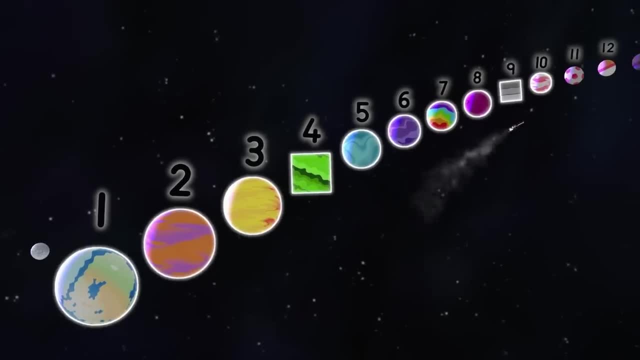 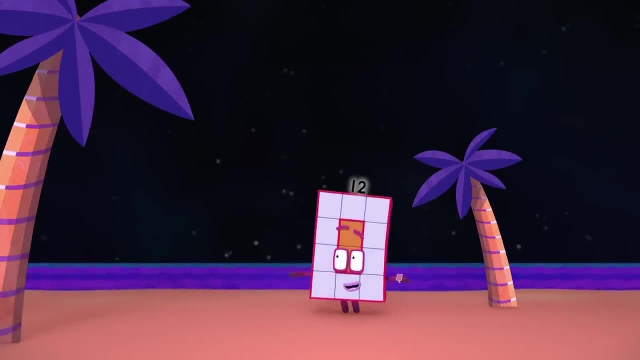 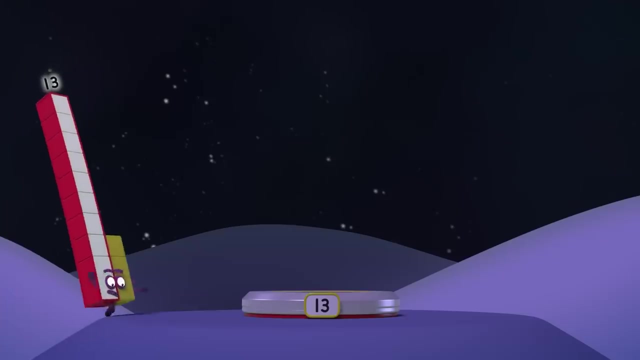 Whoa, Ten planets And one, two more is Planet twelve. Two plus ten descends And one more is to reach a picture-perfect orange beach. Holy Thirteen And off. three pops, Ten steps up and on three hops. 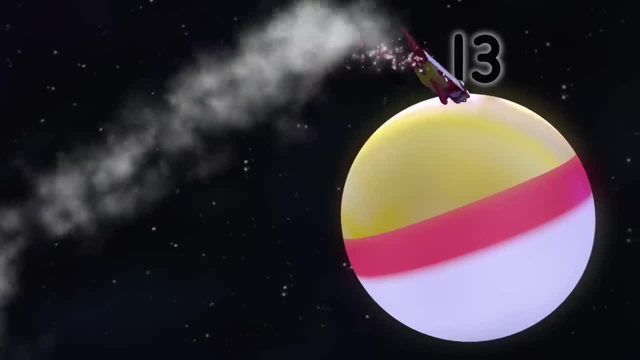 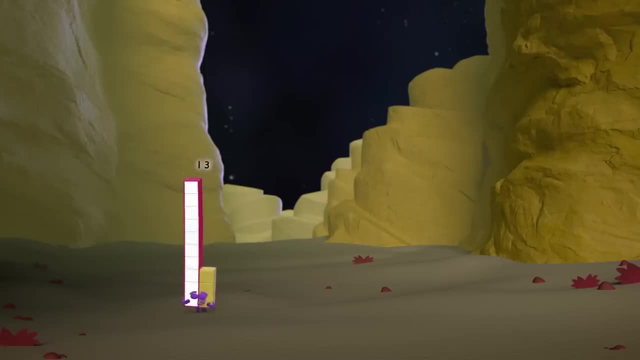 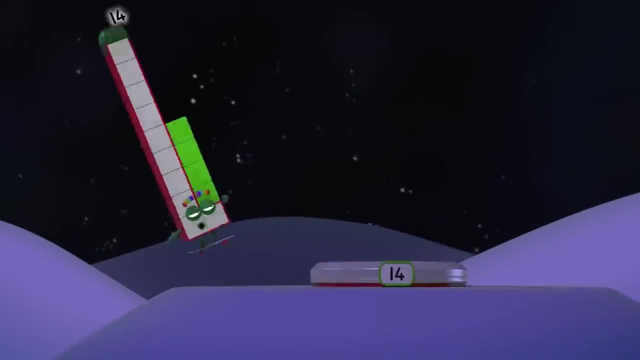 Ten planets, And one, two, three more is Planet thirteen. Three plus ten has found a canyon echoing in wild abandon. Thirteen, Woo, Woo, Woo, Hey, Fourteen gives a big ten. four Ready, steady, off they soar. 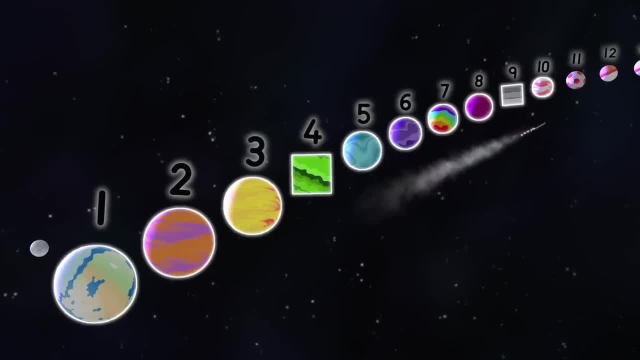 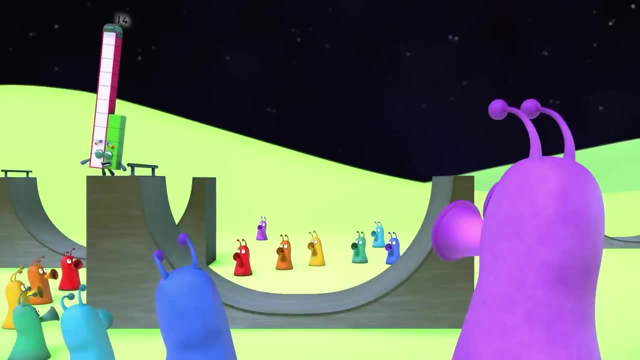 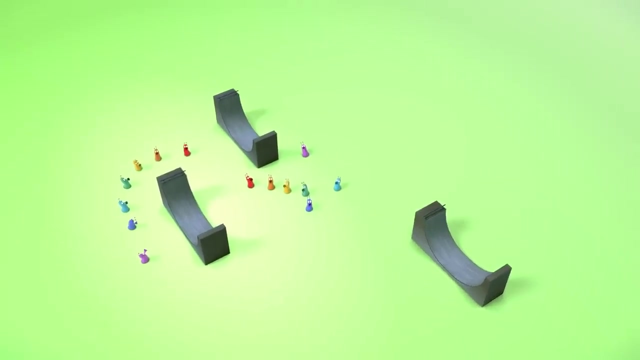 Hoo-hoo, hoo hoo. Ten planets, And one, two, three, four more is Planet fourteen. Four plus ten is full of glee, riding high in zero G, X-treme, Hush, hush. 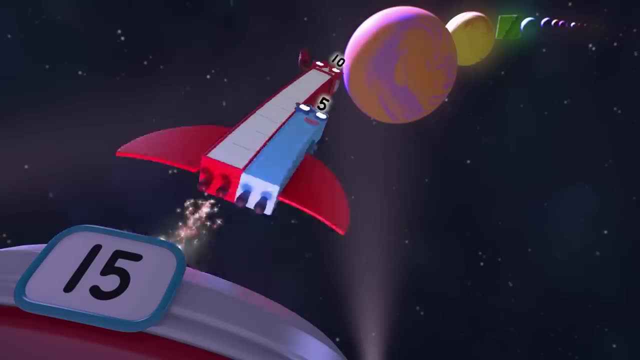 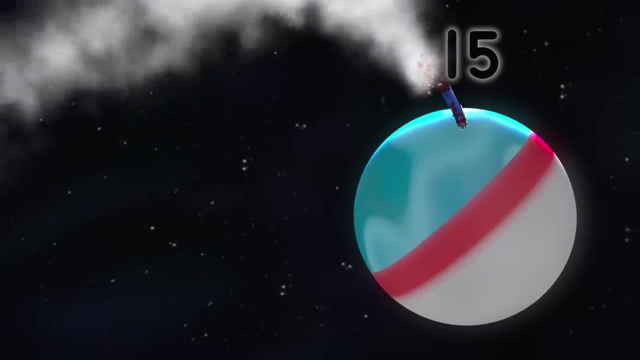 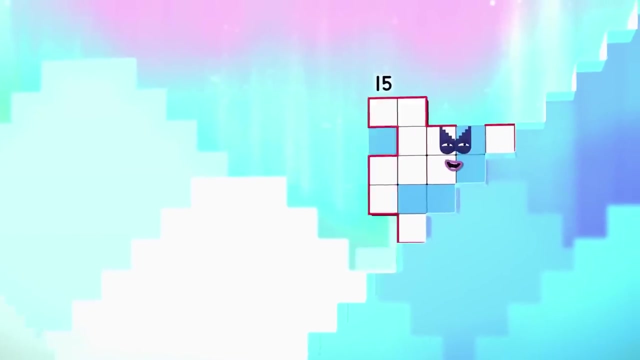 Fifteen is ten and five. Hush, hush, Hush, hush, the rocket roars and off they rush Ten planets, And one, two, three, four, five more is Planet 18.. Five plus ten forgets her cares stepping up the starry stairs. 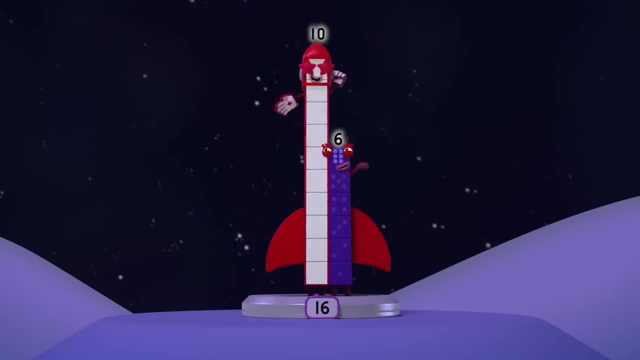 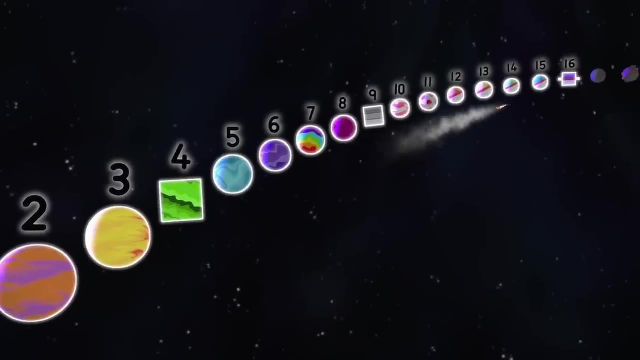 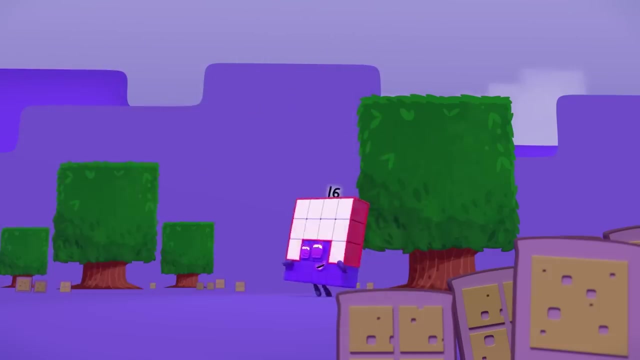 Sixteen squares up to her mission. Ten and six get in position. Woo, Ten planets, And one, two, three, four, five, six more is Planet 16.. Six plus ten has landed where the trees, the cheese, the bees are square. 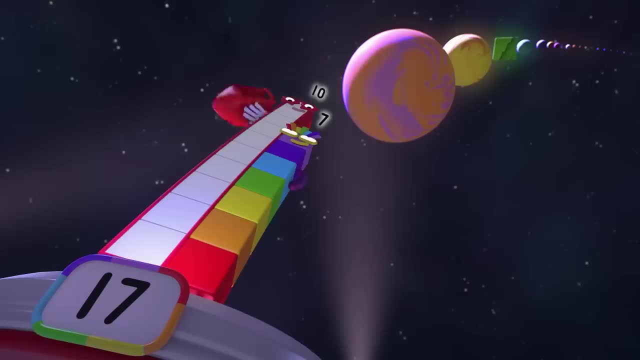 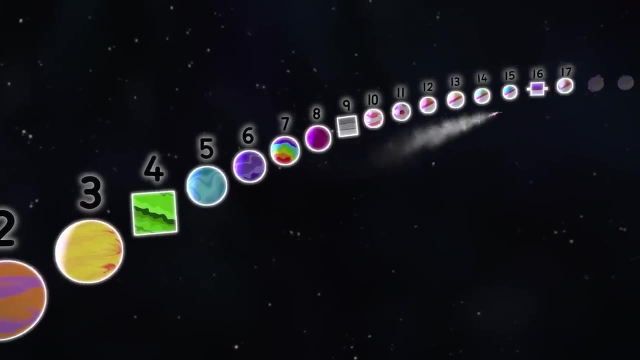 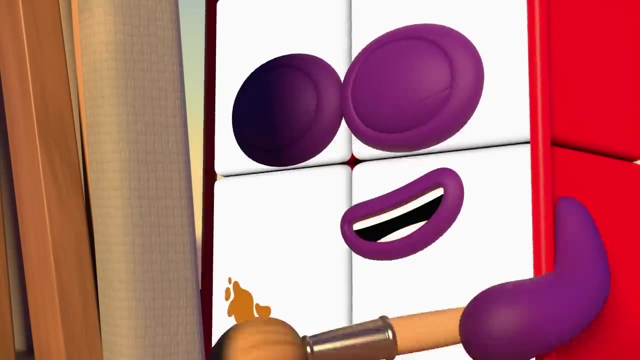 Seventeen must make some art. so ten and seven play their part. Ten planets And one, two, three, four, five, six, seven. more is Planet 17.. Seven plus ten supports, Try surprise, is painting seventeen sunrises. 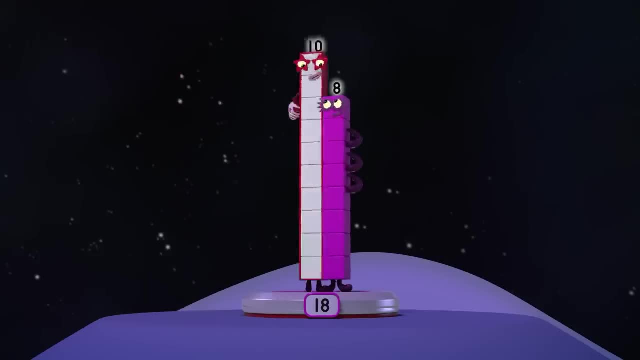 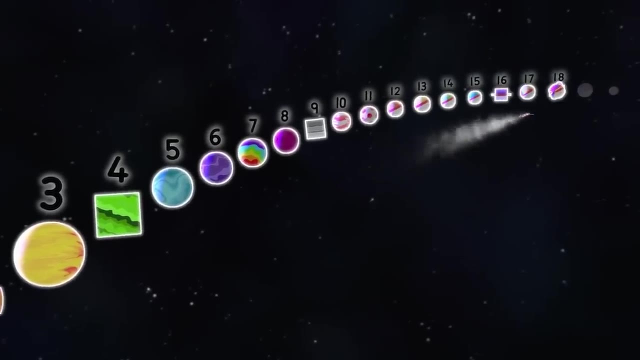 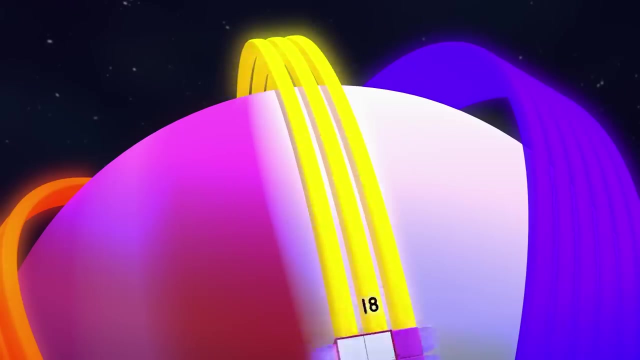 Eighteen feels the need for speed. Ten and eight. it's guaranteed Ten planets, And one, two, three, four, five, six, seven, eight. more is Planet 18.. Eight plus ten is here to race an endless track in outer space. 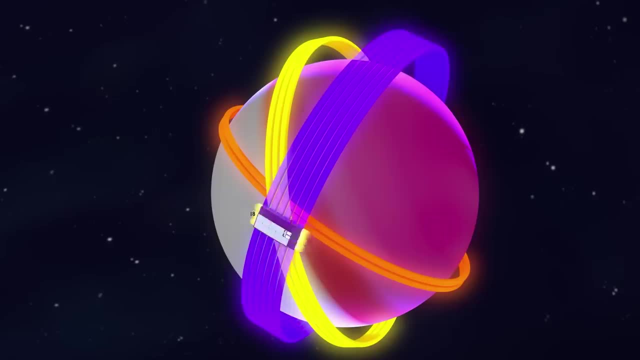 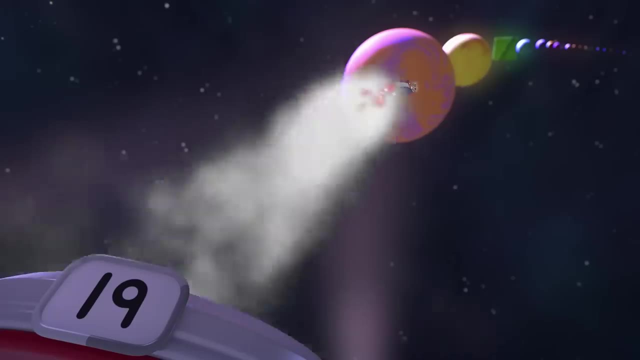 Out of this world. Woo, Woo-hoo. Nineteen, Nineteen's plans are taking shape. Ten and nine make their escape. Ten planets And one, two, three, four, five, six, seven, eight, nine more is. 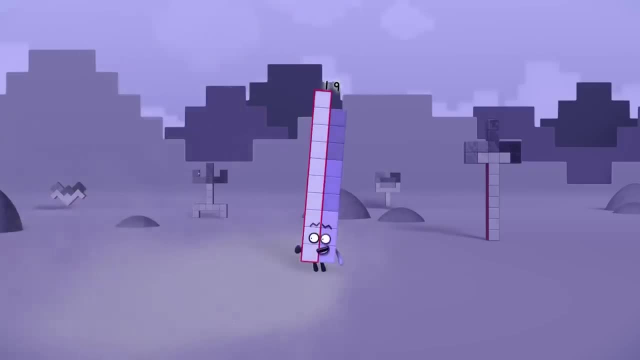 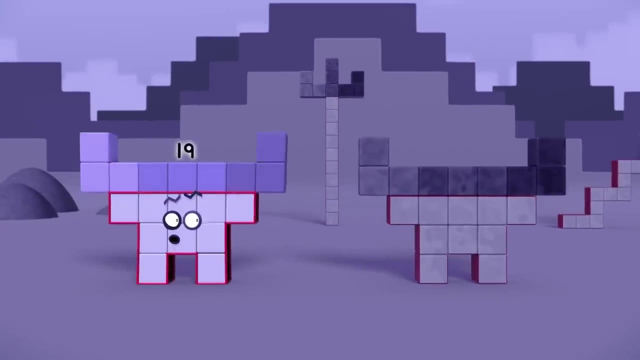 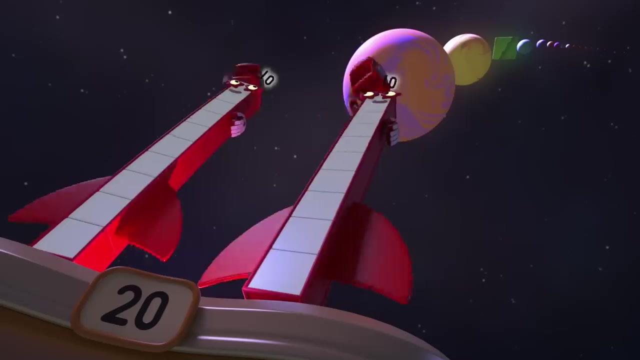 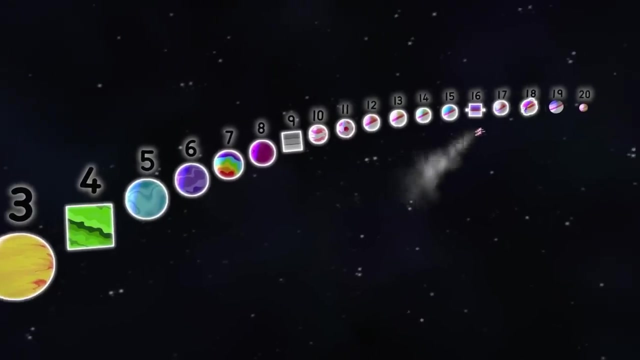 Planet 19.. Nine plus ten is in the flow, with all these crazy shapes to throw. Wow, Cool, Ooh. Twenty won't have any trouble. Ten and ten launch on the double Woo-hoo. Ten planets And one, two, three, four, five, six, seven, eight, nine, ten more is.